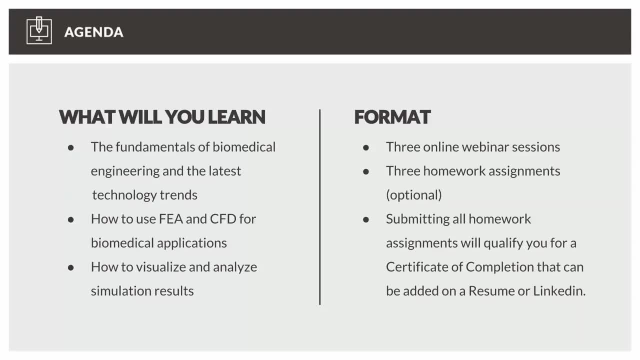 So- And we're also going to relate this to simulation, So let's get started. So, how to use FEA and CFD for biomedical applications. In today's session, we're going to talk about a hip prosthesis. In the second session next week, we'll talk about a stent. 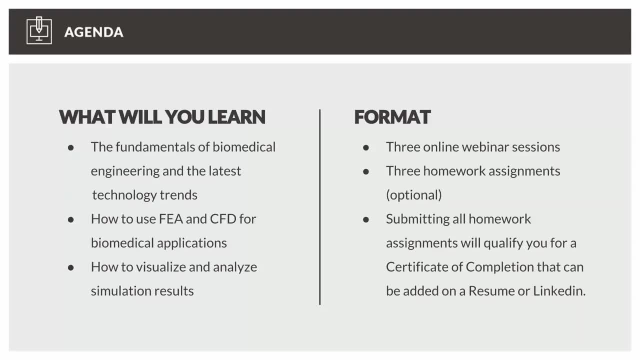 And then in the third session, we're going to talk about fluid blood flow through an artery And overall, we're going to visualize and analyze the simulation results in each session so you learn how to do the simulation and to visualize and understand the results. Now the format of this workshop is a series of three online webinar sessions, one each. 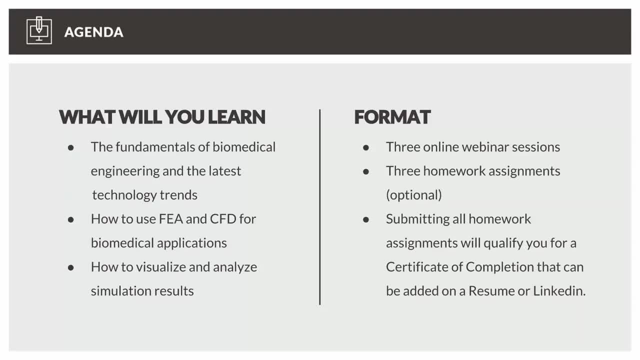 week There will be three associated homework assignments. These are optional, But by doing the homework we feel that you really learn how to apply what you've learned in these sessions And you will qualify for a certificate of completion for the course, and this can be. 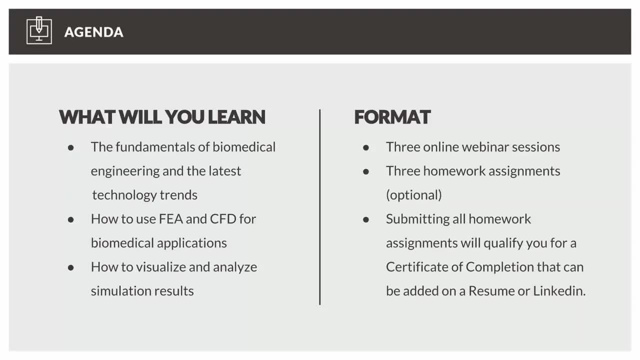 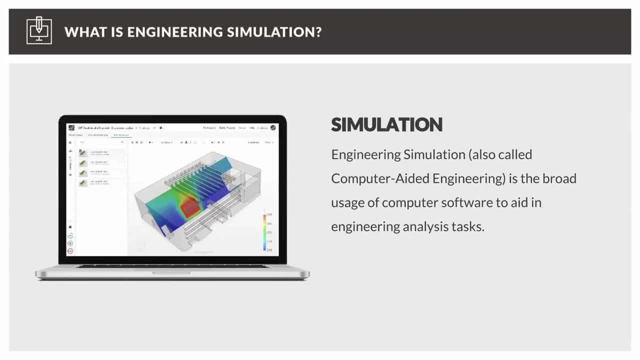 added on a resume or on LinkedIn, All right. So what is engineering simulation? Engineering simulation, it's a very broad term, but it's a usage of computer software to aid in engineering analysis tasks. So just like we have CAD, so we have computer aided design, where we can draw our models. 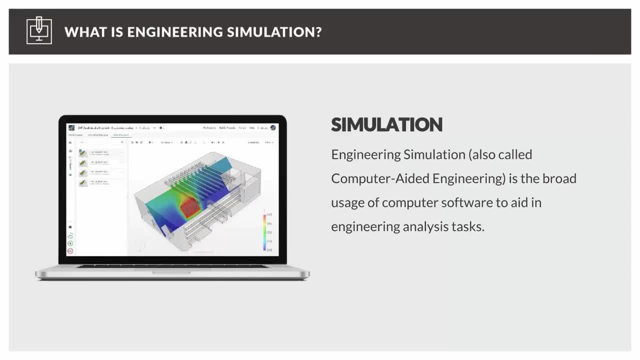 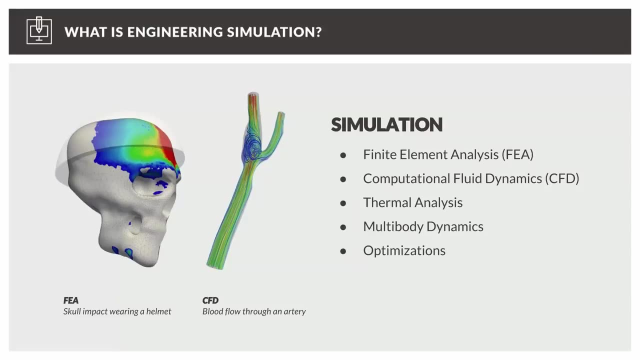 We also have computer aided engineering, where we can analyze and test our models in a virtual environment. There are a number of subsections to simulation, So we have finite element analysis, which is where we want to look at the stresses or displacements. So, for example, we have a skull impact of a bicyclist wearing a helmet. 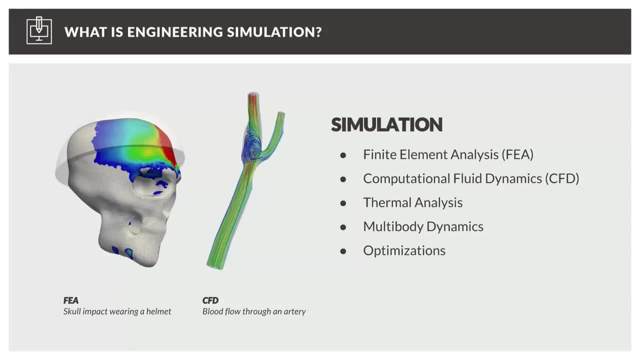 We can better understand how this helmet is protecting the skull and also what forces are going to be acting on the skull, on the skull in the in the case of an impact. The next branch is computational fluid dynamics, so CFD. An example of this would be blood flow through an artery. 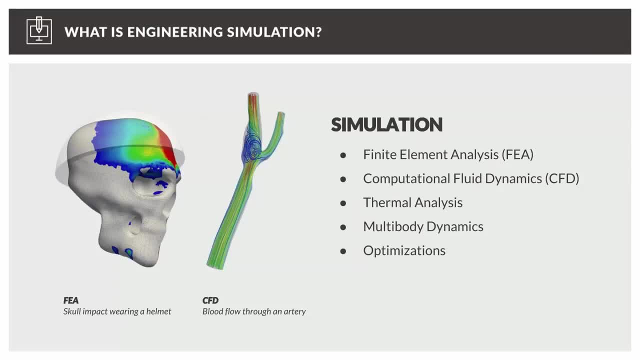 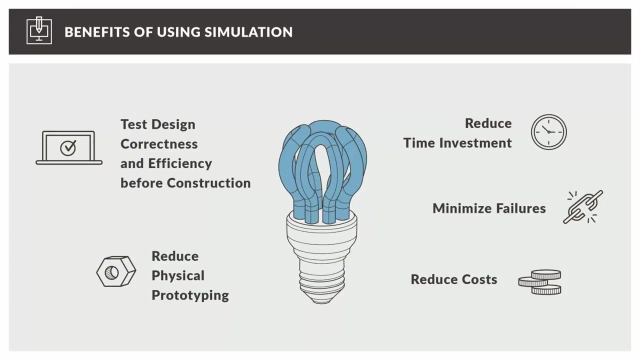 which we'll talk about in session three. And so finite element analysis and computational fluid dynamics. these are the two, the two big topics, and then smaller topics include thermal analysis, multi-body dynamics and optimizations, And in this biomedical workshop we're going to focus on FEA and CFD. Now let's 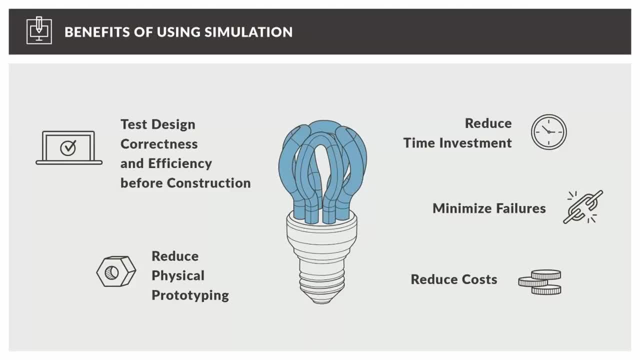 just quickly go through the benefits of using simulation. We're not just using simulation for fun. there's really a big benefit to it. It reduces the time it takes to design- you know, for example, a biomedical engineering device. It reduces the number of physical prototypes. 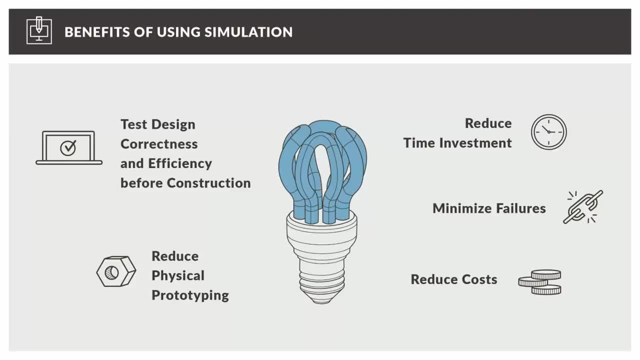 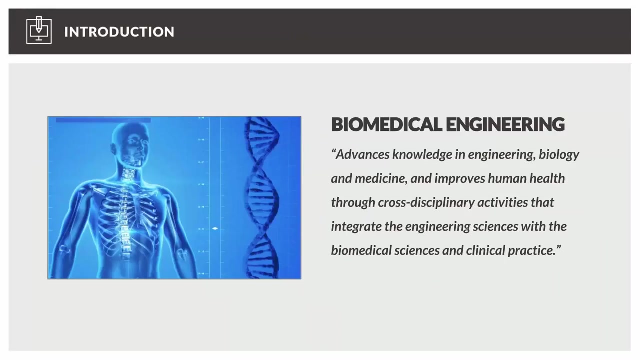 that you need to build, which also reduces cost, and you can really virtually test your design before you build anything. so you can test the design, you can see if it's correct, you can see if it's efficient before you build anything. so it's a very useful. it's very useful in the early design phases. great, so that. 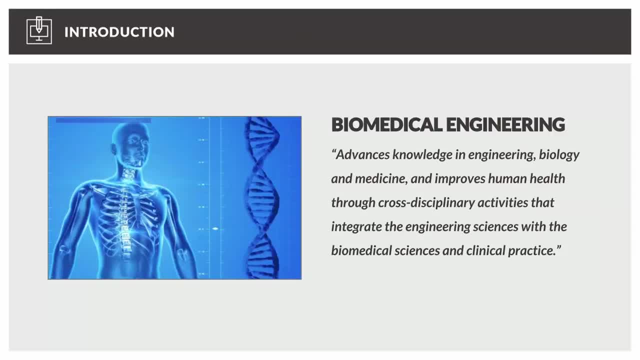 was the introduction to engineering simulation. now let's go into what biomedical engineering is, and here on this slide you'll you'll find a definition of what it is. but I think the main thing to point out is biomedical engineering is really it's a broad field, but it's also very cross-disciplinary. so 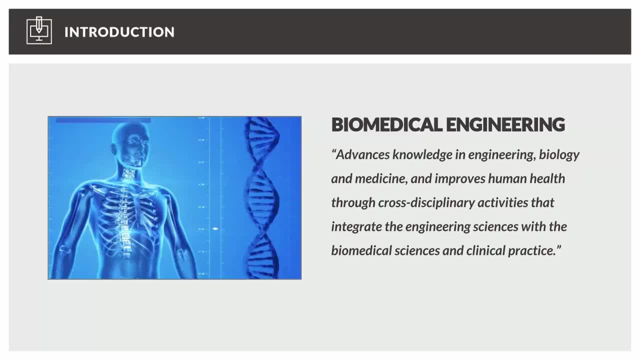 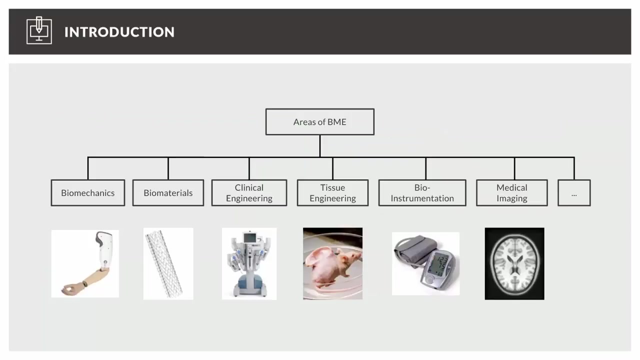 you have doctors, biologists and engineers who are really working together to figure out ways to improve human development and how to improve human development and how to improve human health, either through technology or prosthetic devices, implants and things like that, and so let's talk. let's now talk about the areas of biomedical. 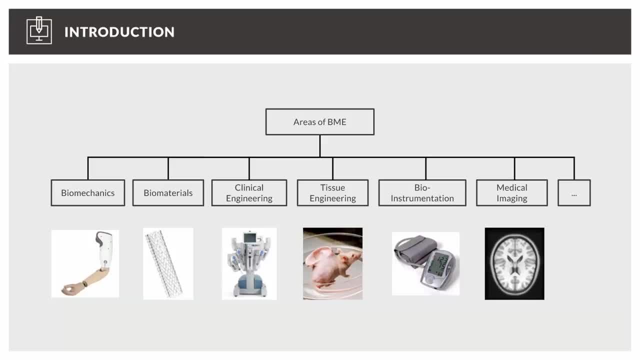 engineering. so again, this is very broad. we can start here with biomechanics, which is kind of what we're going to be looking at today. this is more more engineering, I would say more similar to mechanical engineering, but biomechanics would involve any sort of implants or prosthesis. so today we're 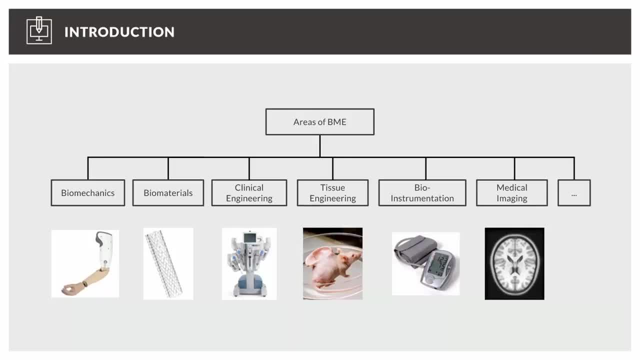 going to talk about a hip implant. then we also have biomaterials. so, especially for medical applications, biomaterials obviously need to be non-toxic and they need to work well within the body and not be rejected by the body. clinical engineering, tissue engineering- so here. 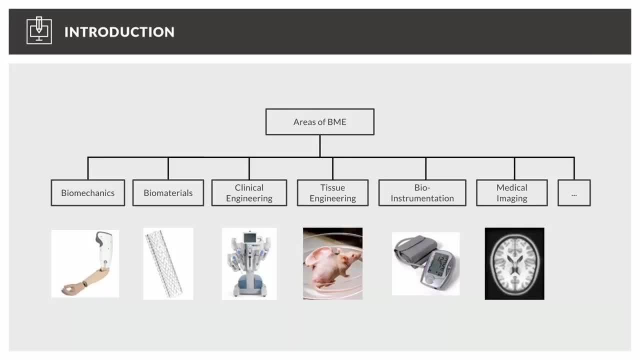 you can see a rat that has an ear kind of growing on it. so different applications here. this is more, more maybe biology type applications, bio instrumentation and medical imaging. so medical imaging would be your MRI, CT scans, x-rays, things, things like this, so not actually things that are in the 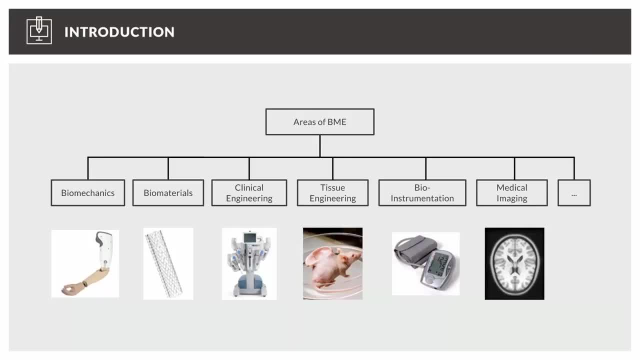 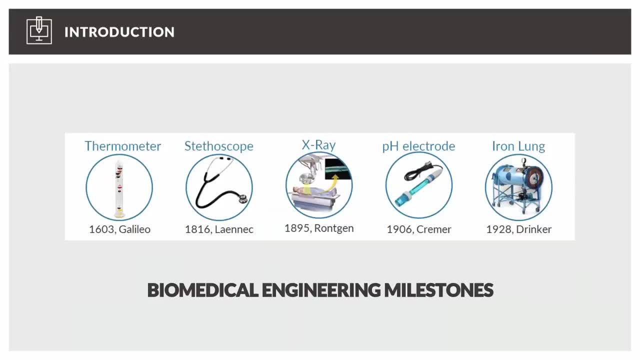 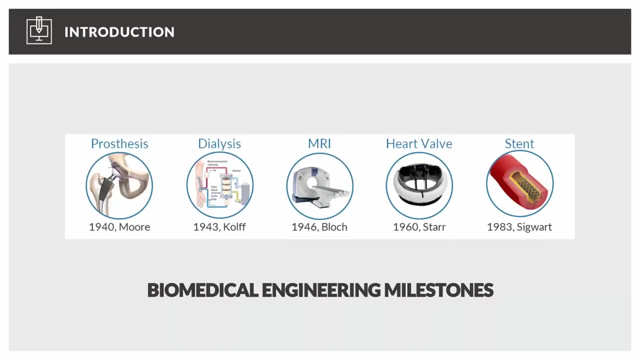 human body, but applications that help us to understand the human body better. another piece that's more important is ethnicity, representing the ways in which people get vaccinated and how raus て the iron lung and, even closer to today's times, this prosthesis hip implant has. 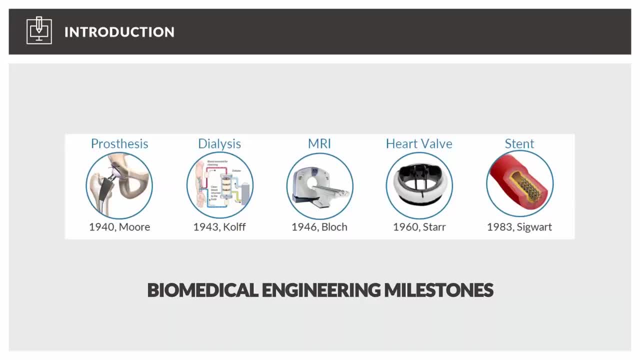 was developed in the 1940s. this is becoming more and more common for people that have problems with their hip getting these, these type of implants. it's safe, a safe technology nowadays: dialysis, so the ability to clean the blood if the kidneys don't work correctly, heart valves, stents, things like. 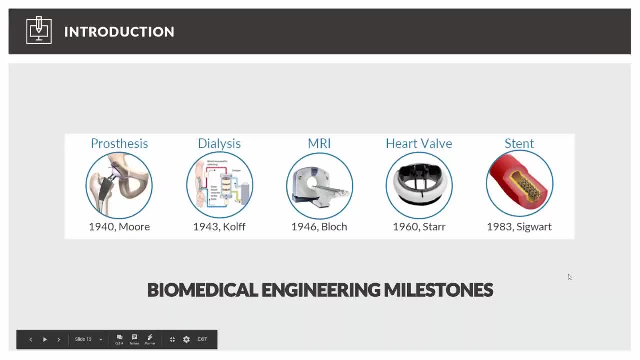 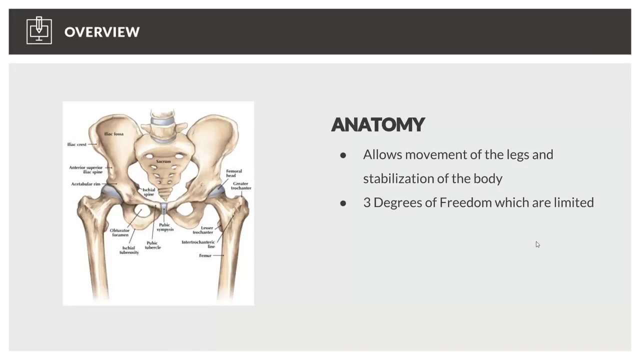 this and so in in this biomedical engineering workshop, we're going to focus on three of these applications: the prosthesis, blood flow through a heart or an artery, rather, and this stent design. so now let's go in today's, into today's topic, which is hip. 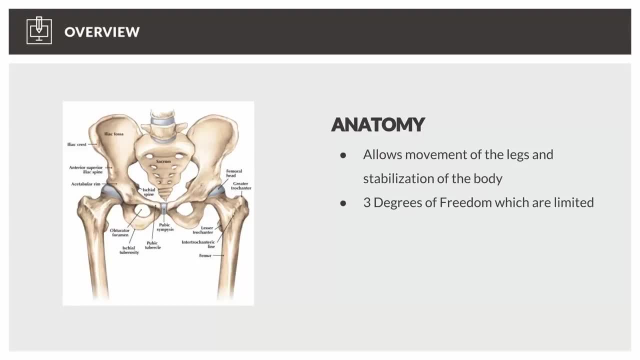 replacement. we're going to talk about a hip implant and let's start with just talking about the anatomy of a hip, of the hip. so, basically, what the hip is doing is it's allowing, you know, it's attaching your leg, your legs, to your body. it's allowing movement of your legs. 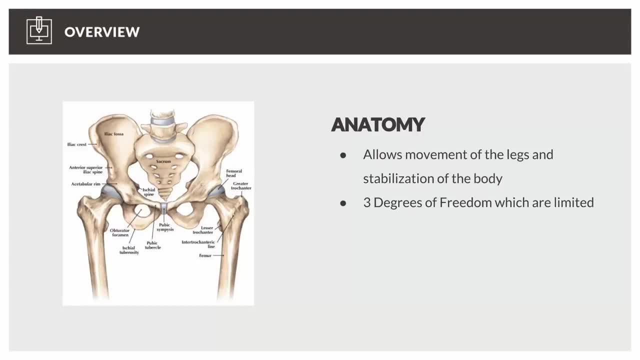 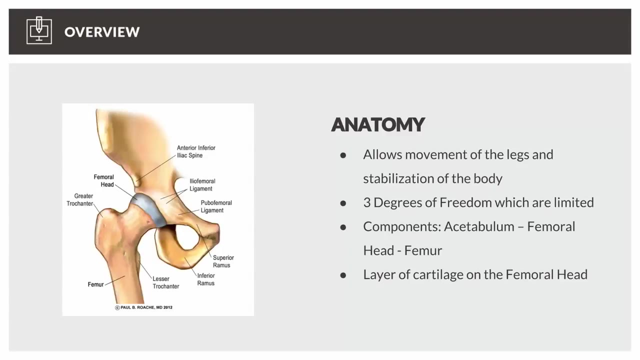 it's giving you that three degrees of freedom which you enjoy. obviously it it's limited, so it's not a full range of motion and as you get older that range of motion will decrease. if we go in a little bit closer, we can kind of get a. 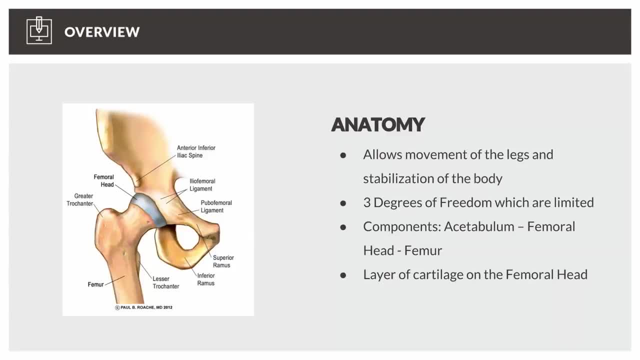 better view of what it looks like. so we have the femoral head which is there's a layer of cartilage there which kind of allows the hip to rotate smoothly. so this is connecting to your, your femur and your, your pelvis, which is giving you 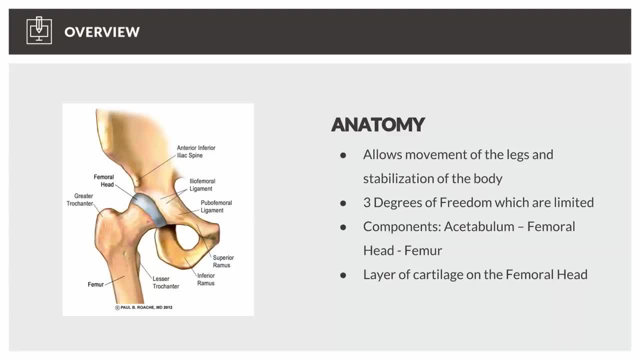 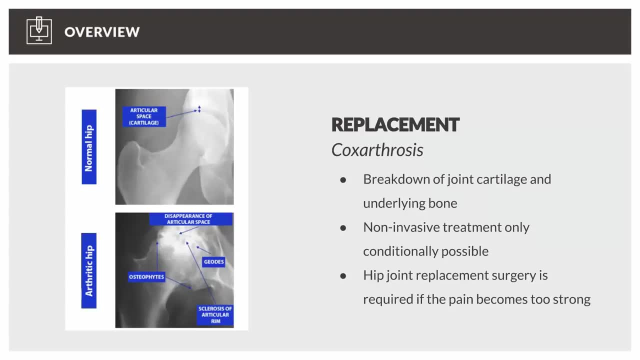 that, that range of motion that allows you to walk and jump and run. now, in some instances this can be an athletic injury, maybe from playing football or just aging. you can sometimes get a breakdown of the cartilage in this hip joint and if it becomes very, very painful, sometimes it's it's necessary to have a hip joint replacement surgery. this is kind of a last, last-ditch effort. there's a lot of non-investment in non-invasive treatments. that can be done first, but once the pain becomes too much and and there's no more non-invasive, non-invasive treatments, then it's time. 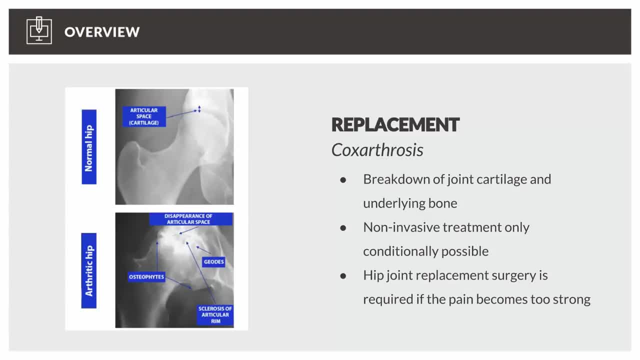 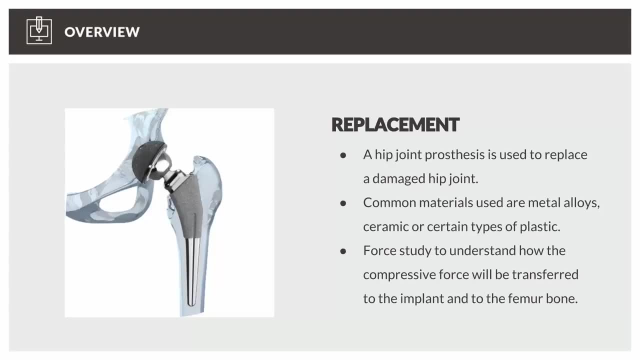 to do the hip joint replacement surgery, and so this, this is a. this is an image on the left of a hip joint prosthesis, and this is what is. this is what's being used to replace a damaged hip joint. generally, these are made out of either metal or certain types of plastic, and 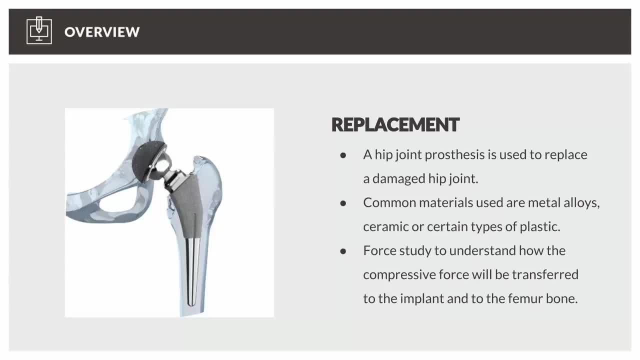 ceramic it. it kind of depends on the model that you're using and what we can do and what we're going to do. is we're going to do? is we're going to do a today's session? is we're going to understand how the forces are, what, what? 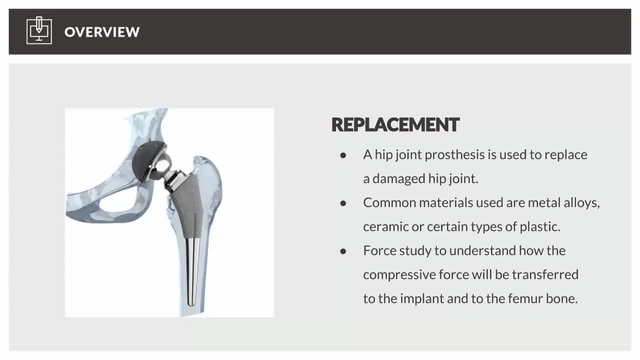 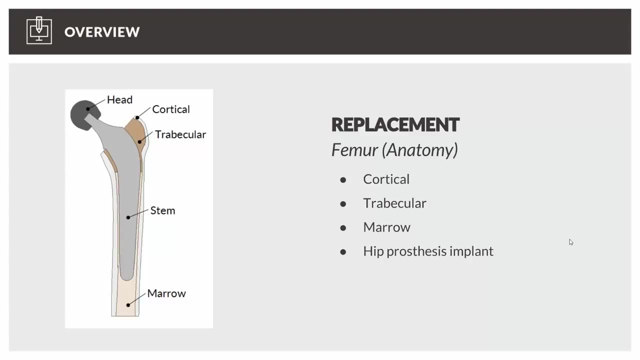 forces are being applied to this hip joint prosthesis and how the and how those forces are being put on the bone or the femur. and let's get a little bit closer. look at the replacement anatomy. so again you can see the implant here on the left. 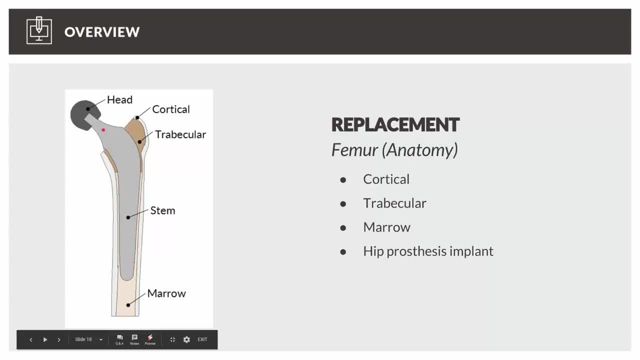 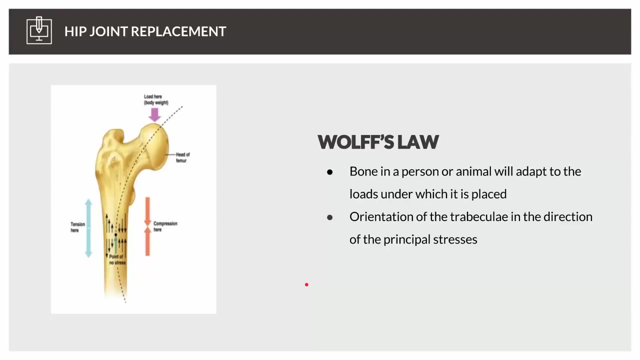 maybe I can use a pointer so you can see here this is the implant. so sorry, this is the implant stem. and then there's a head and then we have bone around this. so we have the cortical bone, trabecular and then bone marrow here. now the way the the load moves. 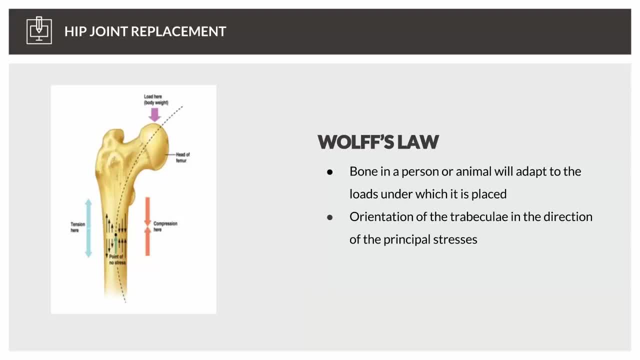 through the body is is quite interesting, and this is a known as wolf's law. so, basically, what happens is when loads are applied to your body, your bones will adapt. so if the loads somehow change, if the weight of your body changes, your bones will adapt to different loads, under which that's placed, and and what. 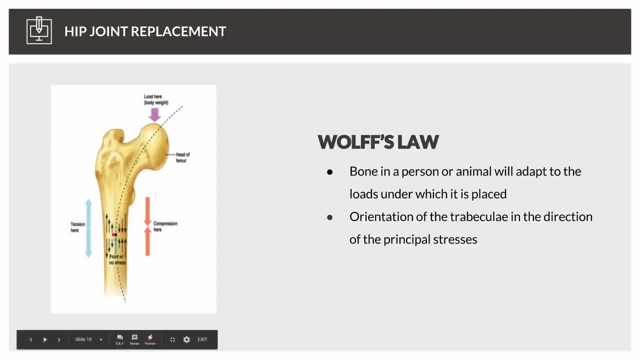 it's doing is. you can see, here we have normal stresses. generally, the body load is applied directly on the hip, and so on this side of the bone we have compressive stresses and on this side of the bone we have tension stresses, and this will be important. this, this the way. 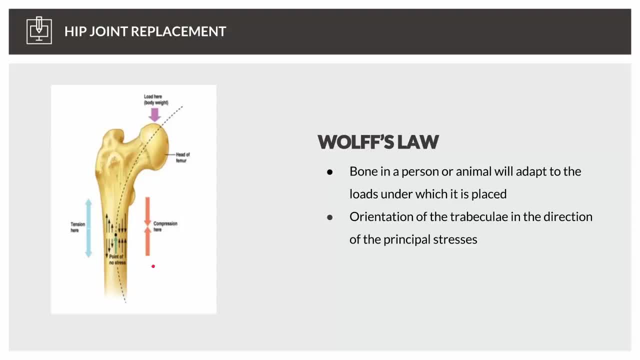 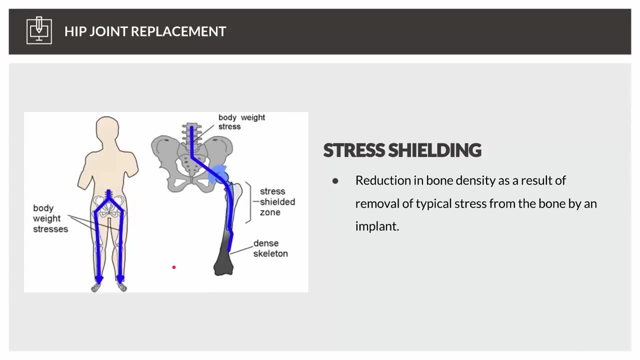 the way the forces move through the bone will become important later when we look at the results and and basically, what can happen is if you, when you have a normal, but when you have your, your normal layout of the body, the stresses are equally distributed on on this, on this bone, this femur bone, and 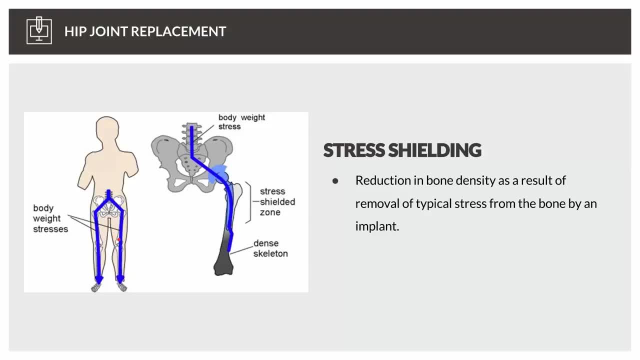 your and your body will obviously adjust. so the the density of the the bone in your body is adjusted to how how the load is. but what can happen is when you have an implant, as we see here, it changes the load path and so more of the load. because we find that these implants are, if they're made. 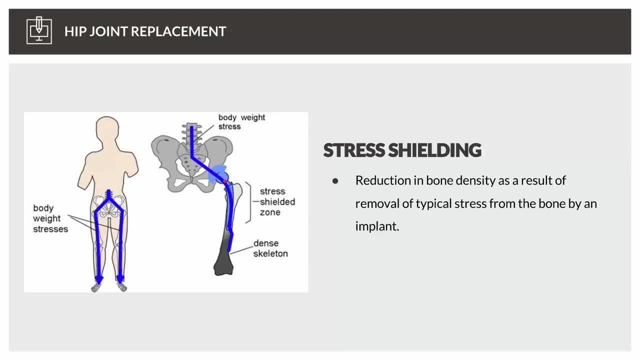 out of metal, for example. they are stiffer than bone, and so more of the load will be absorbed by this implant and less will be going to to the actual bone itself. and so we get this thing, this, this concept called stress shielding, and this is the reduction of bone density as a result of stress. 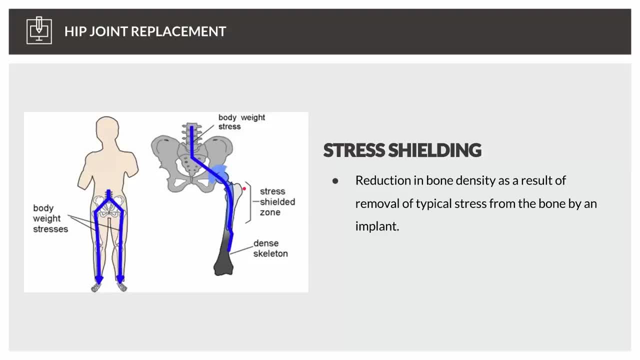 being removed from the bone, and this can happen, and this does happen with with implants. so more, more of the, the compressive force is being taken by the implant and less is being passed on to the bone, and so the bone starts to weaken and and loses strength. so you actually will start to lose bone in your 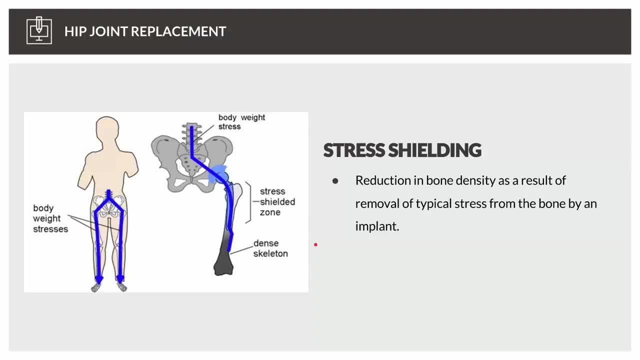 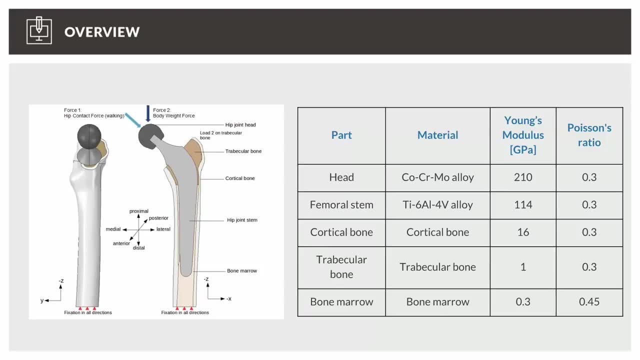 leg. okay, so we just discussed stress shielding, and so now we're going to go into our main application topic today and I'm going to describe a little bit of how the setup works. so, again, we can see our bone, and then so we have the, the main, the main thing to focus on here. 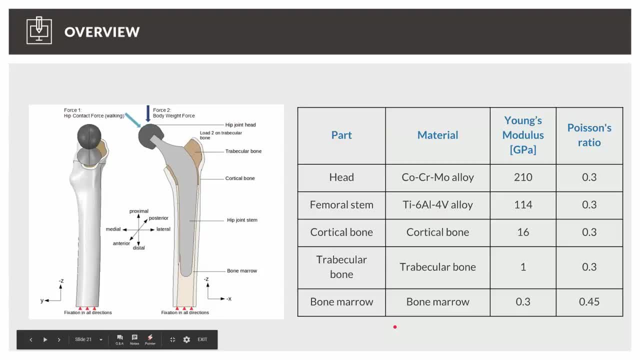 is the materials that are being used. so the implant, in this case, will be made out of metal. it's going to have the head will be made out of cobalt, chromium alloy, the stem is going to be titanium, aluminum alloy, and then these bone structures will have different, varying properties, and so it's important to 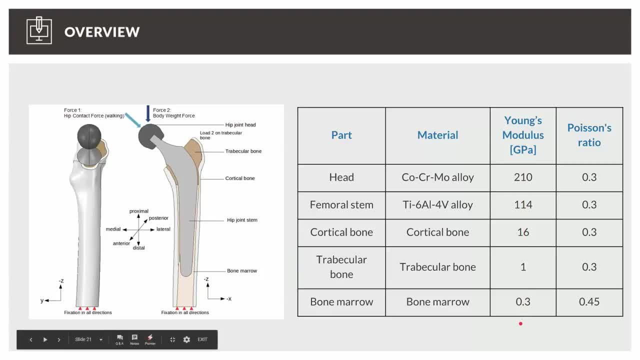 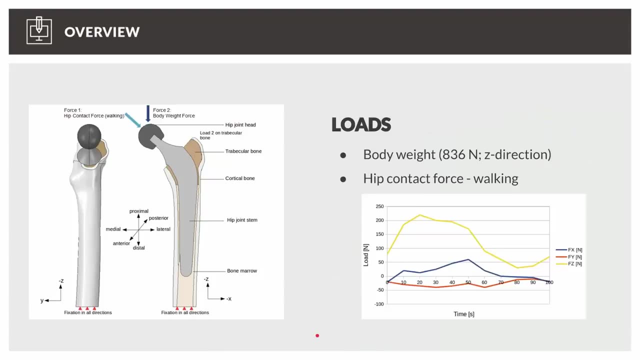 notice that obviously here we have the young's modulus, and this is a. this is a factor of stiffness, and so you can see here that the metal alloys are are very stiff compared to our bone structures. and the second thing to talk about is the boundary conditions of how, how we 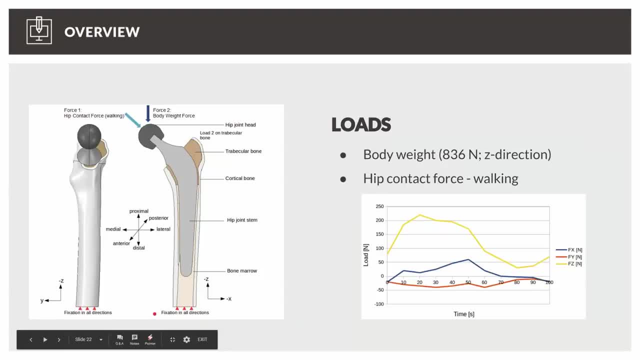 how we look at the loads on this. so we basically have it fixed at the base and then we apply loads here on the head, and so force one is a hip contact force. so this is the forces on your hip when you're walking and we can actually see. 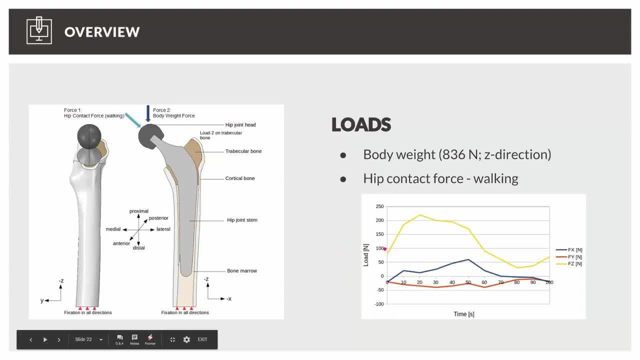 these here in this graph, the variation of how, how the hip, or how the force is applied on the hip due to walking. so that's the first, the this force number one. force number two is a constant load. it's the body weight of the person. so around 836 newtons for an average human would be a the weight. 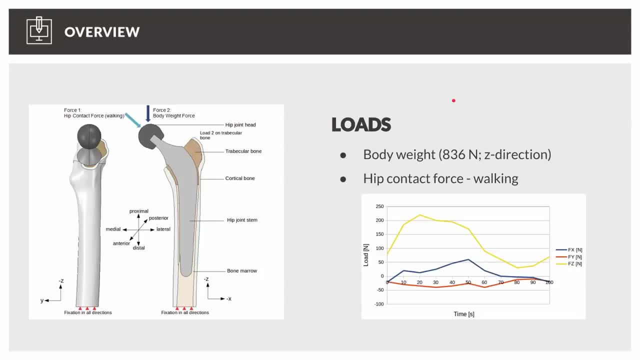 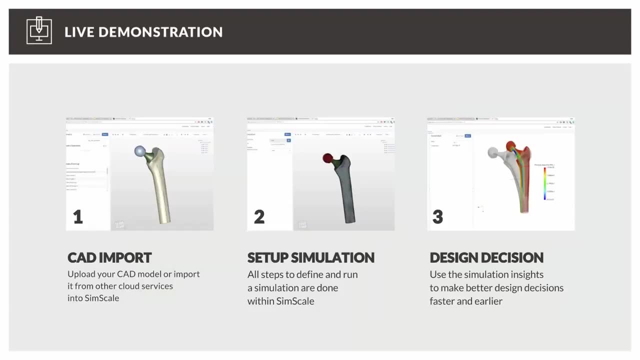 that will be applied on this. this hit ok. so those were the main. that was the main theory that will be covered, and now we're going to switch over to the live demonstration, and so first I want to talk a little bit about how the simulation setup works with these three steps. so the first thing that that we do, 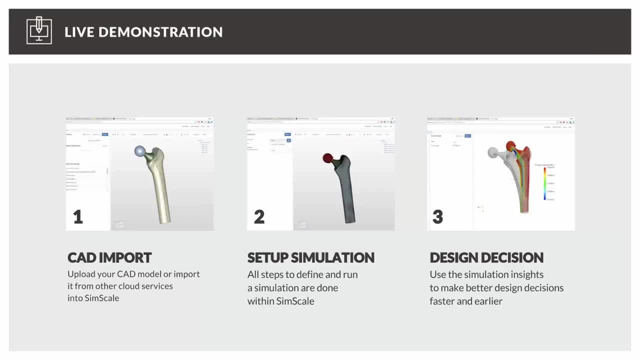 on the same scale platform is you need, and when you do simulation in general, is you need, to import your CAD model so you can? I mean this CAD model. I'm not sure where it was generated, but it needs to be uploaded first to the same scale platform. 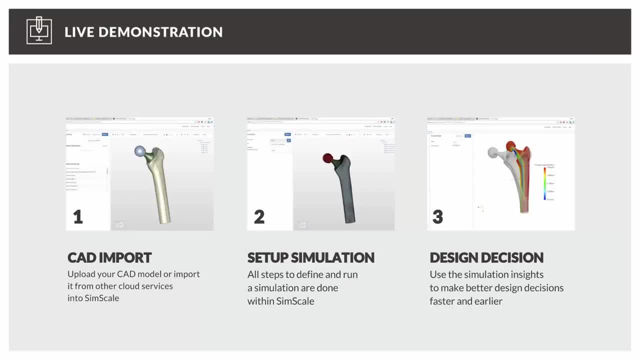 clean and simplified. so removing any small faces or things is the first step. the second step is setting up the simulation, and so that means, just as I showed you in the previous slide, you need to apply your materials, you need to and then apply the loads and the fixed boundary condition as shown, and then, in 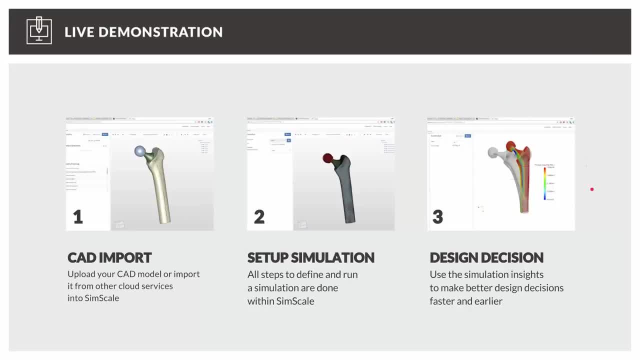 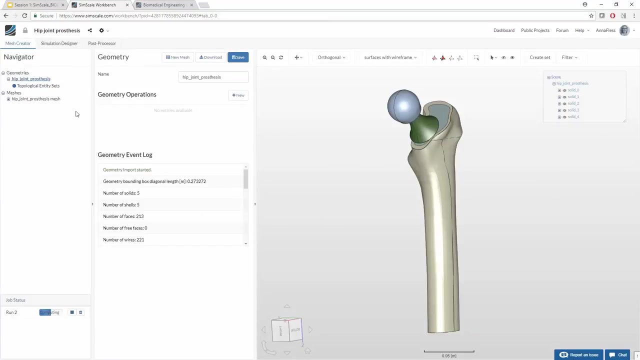 the final step- which this is the most interesting step, obviously- is to look at the results and try to learn. you know how these loads are affecting the hip. ok, so now I'm going to switch over to the same scale workbench, which I hope you can see my screen right now. so this is the same scale workbench as you can. 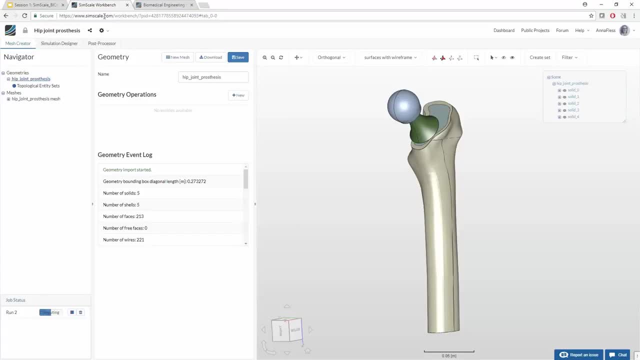 see, I'm working in my my web browser and in the chrome web browser. I'm doing everything online. right now I'm in. I'm in the same scale workbench, so the first thing to do is upload the hip joint prosthesis, which I've already. 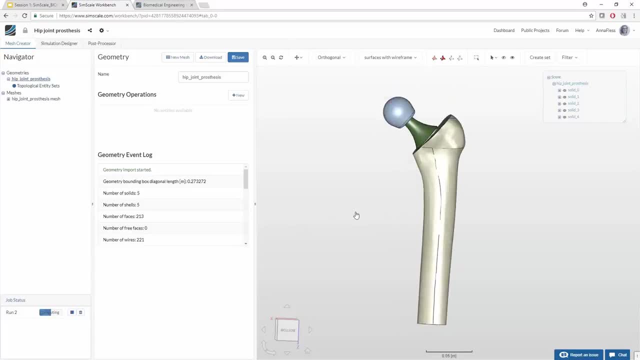 done. I can see it in the viewer, I can rotate it, zoom in and out, and let's have a look at the different solids that we have here so you can see the head, which is solid. for then we have the, the stem here, the implant stem. this is solid three, this is the cortical bone that I 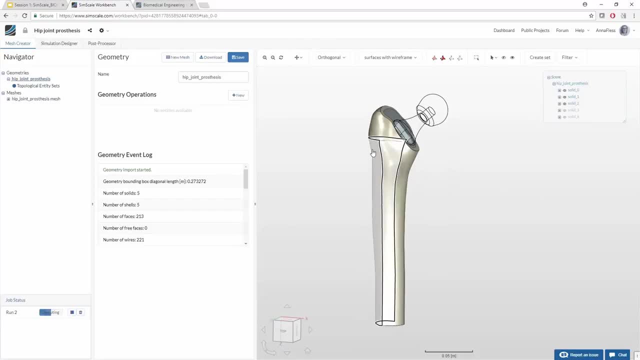 just that I just hid this bone. right here is the cortical bone, then we have in the blue, we have the bone marrow and then finally here, the trabecular, and so there are five components that make up this, this model. and now the next step. what we want to do is we need to mesh this, and so what? 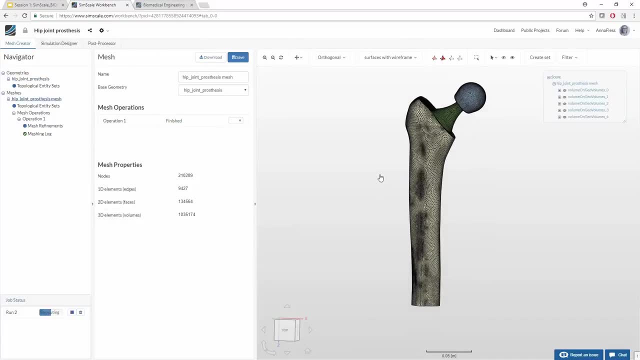 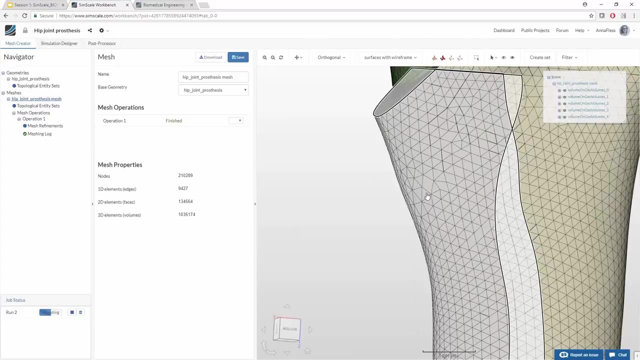 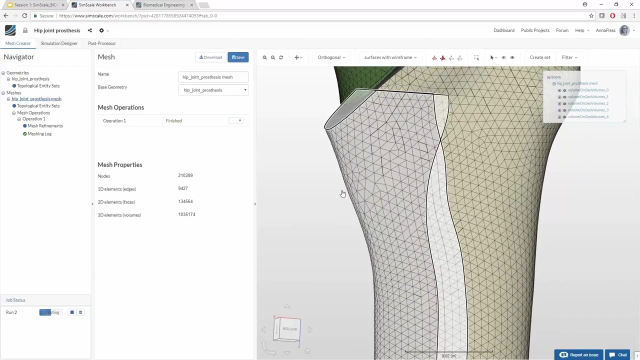 meshing is doing is it's breaking down our geometry into smaller elements, and if i zoom in, you can see all these small elements that that this geometry is made up of now and what. why we do this is because we're we're using numerical methods to solve for the stress and displacement in this case. 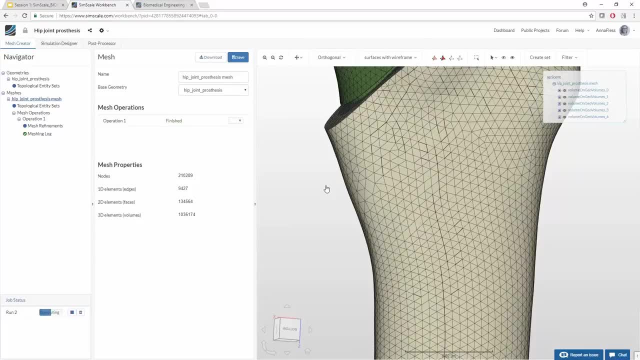 and we can't just do that over the whole body, over a continuous body. we need to break it, it down into smaller elements and we generate a very, very large system of algebraic equations that that can be solved on a, on a computer, and so for each of these elements were solving, for each of these elements will. 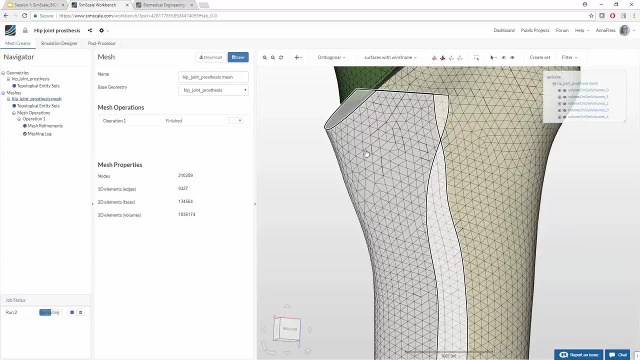 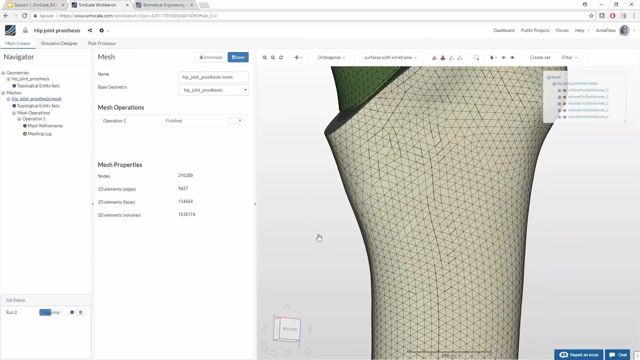 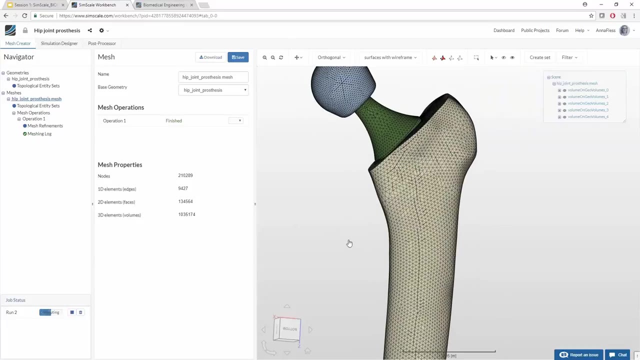 have notes on their, at their, at their, on the points- and this is where we're actually solving for the displacements, which allows us to find the strength, stresses and strains when a load is applied to this model. and just to give you a quick overview. you'll learn all this in if you do the step-by-step. 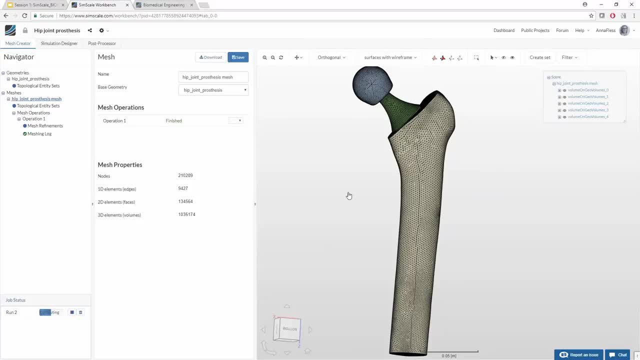 tutorial and the homework that it will be shared with you later you'll you'll get to set up this up by yourself. so I'm just going to kind of do an overview of how the steps work. I'm not going to fully fully show everything, but if I go, 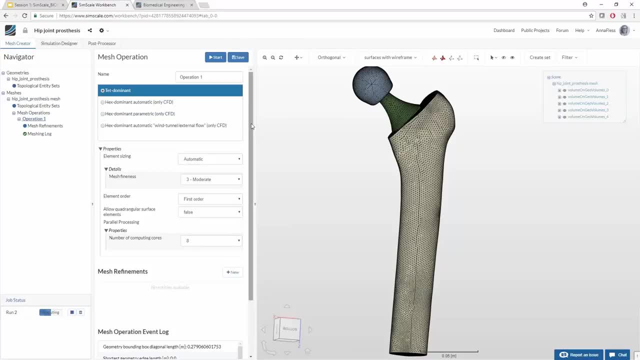 to operation one, we can see the settings for this mesh. so this is a tet dominant mesh, which is generally what we're using for finite element analysis, where we're trying to solve for the stress and the strain I'm using in the automatic meshing algorithm. Simscale has this, so it makes it very easy to 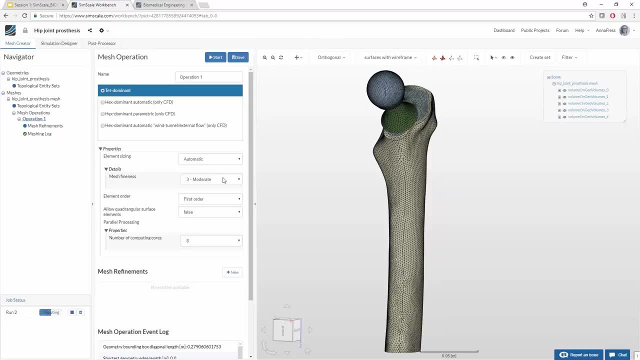 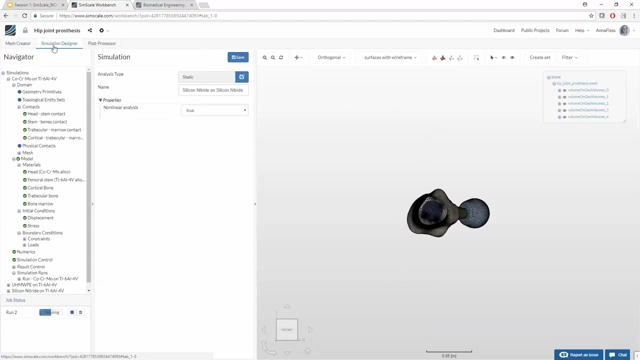 create a nice mesh- moderate fineness- and then I'm using eight computing cores to solve for this, and so this mesh, I created this in about five minutes, I think. so that's all the time it took. so now, once the the mesh is complete, the next step is to set up the simulation, which is what I'm going to. 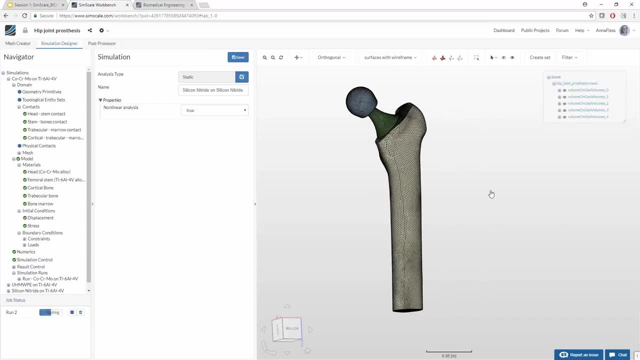 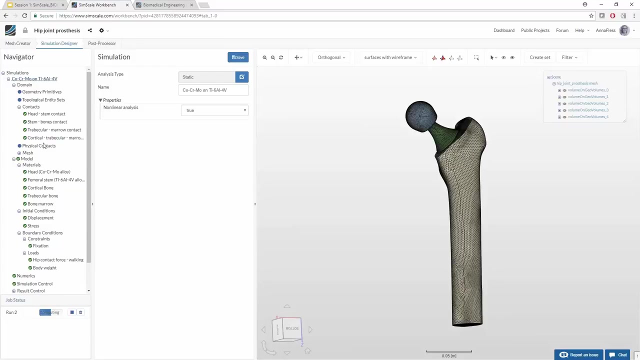 show you right now, and so, basically, what can be done is you're provided with this tree, so it gives you all the steps that you need to fill in, and it can look a little bit overwhelming, but it's quite easy once you go through it. it really if you click on every single. 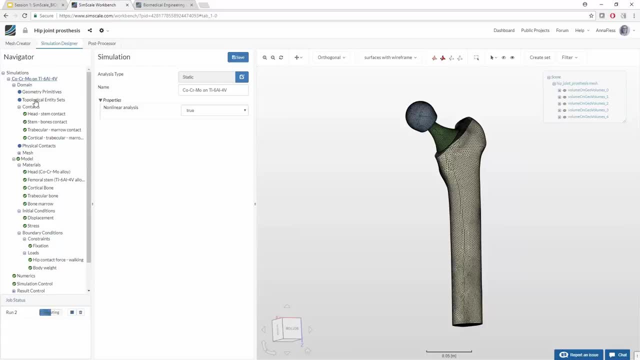 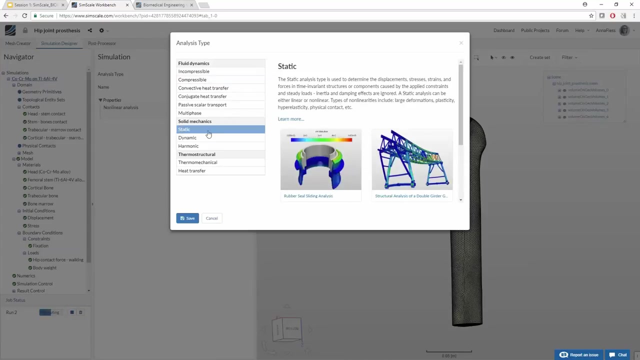 item in this tree and you fill in the information, then you've correctly set up your model, and so the first thing that needs to be chosen is the analysis type, which in this case is static, since we're just applying and we can have a look here. so it's nice in Simscale, it gives you a description of what static is. so 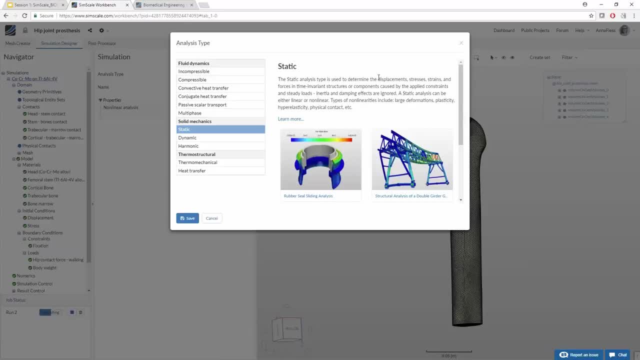 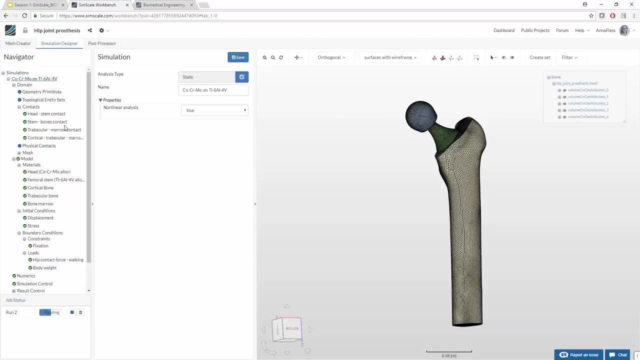 in this case, we want to determine the displacements and stresses on this structure, so we're going to use a static load or a static analysis type. now the next thing that we need to talk about is contact. so, as I showed you earlier, this model has five it's contained of. it contains five. 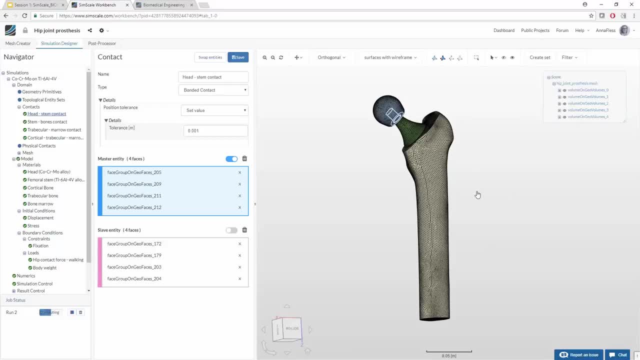 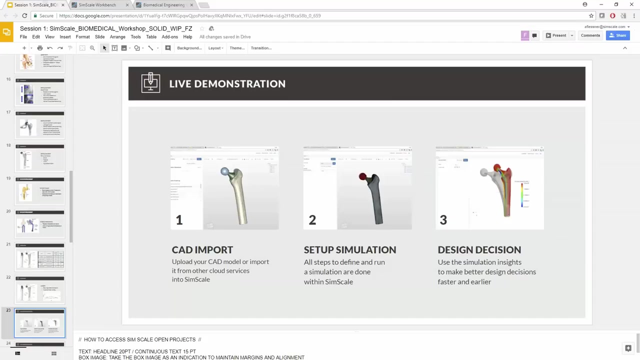 different solids and on Simscale and when you're doing FEA, the solver doesn't know that these volumes are connected to each other, unless you tell it that they're connected to each other. so we have to set up, we have to set up the contacts and I have this actually in my slides. 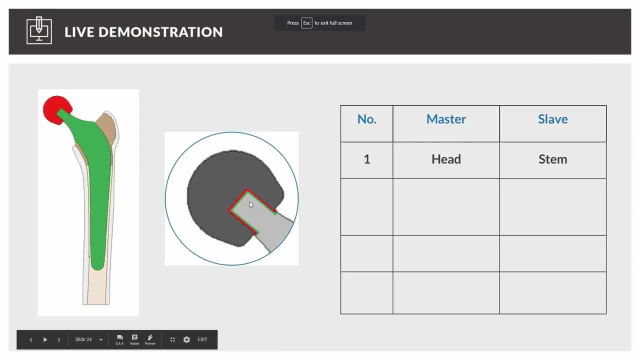 which might be easier to see, and so this is what we're doing. so if we first look at the implant stem in the head, we can see here that we need to attach the contact. so these faces of the head need to be attached to these faces of the 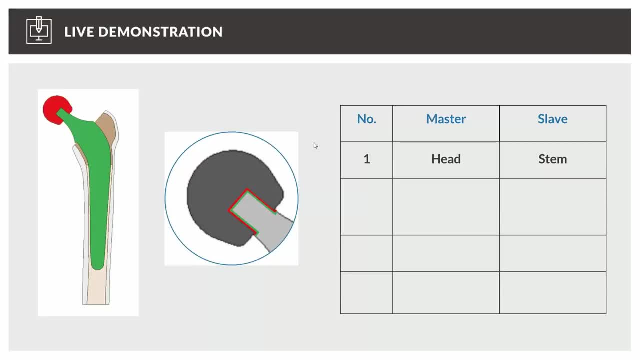 stem, and we'll do this by using a master and a slave face. so, basically, what the master face is doing is the master face all the nodes. when those nodes move, they're connected to the slave nodes, and the slave nodes must follow the movement of the master, and so that's how these contacts are working. 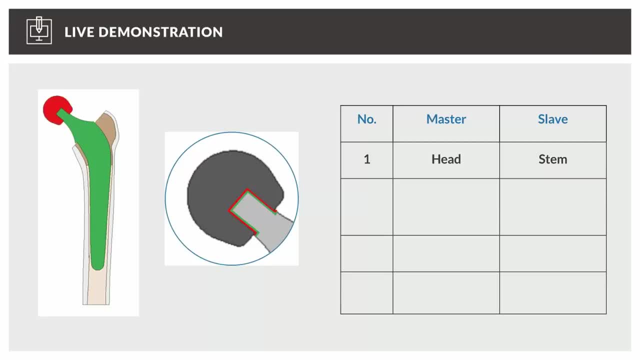 and right now we're setting up contacts that are that are bonded contacts. so it's basically like we're gluing these two components together and we're going to do this for the remaining of of the faces. so we have to make sure all the parts are connected. so the first is the head in the stem and now we can see the 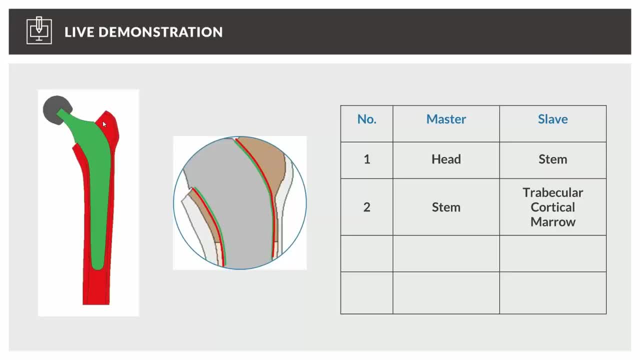 stem also needs to be connected to the trabecular. here maybe it's easier to see here. so the stem needs to be connected to the trabecular and part of the marrow here all the way down into this section. then we have the trabecular and the marrow, so get the pointer again. so this red section. 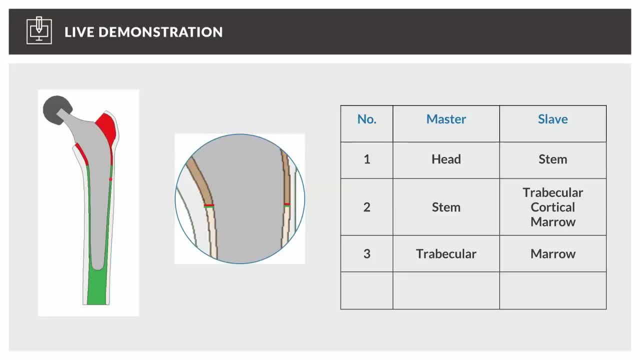 here needs to be attached to this green section, which is the marrow, and we do that at the interface where they meet. so you can see, here, this is where our contacts will be set up. and then, finally, the marrow and the trabecular need to be connected to the outer bone, the outer cortical bone, and so, with all those set, 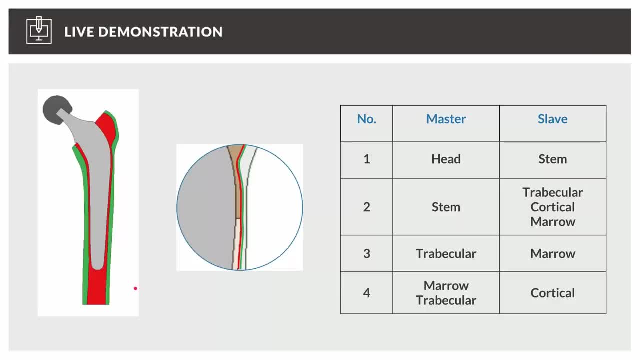 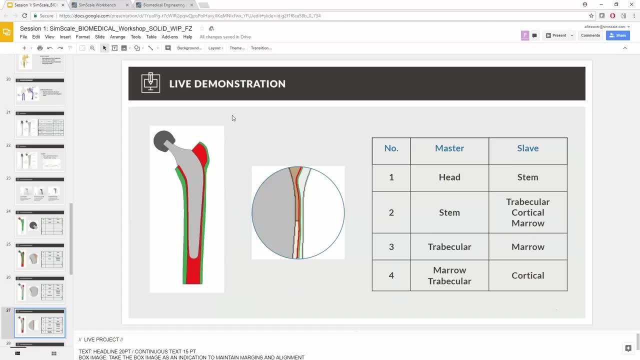 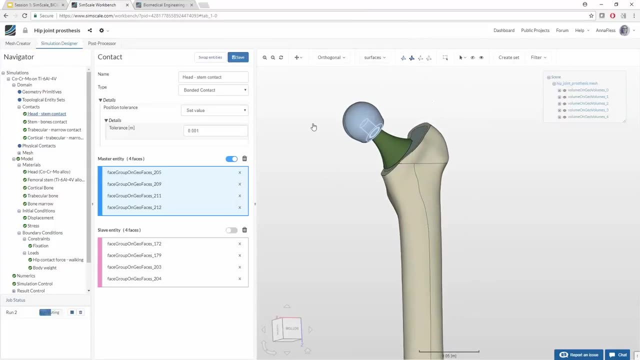 up. our whole system is connected, everything is glued together, and now our solver knows that we want we want everything to be connected, and so if I go back to the workbench, we can actually see this as well. let me change this to surfaces. so if I zoom in here, you can see the master faces of the of the head are. 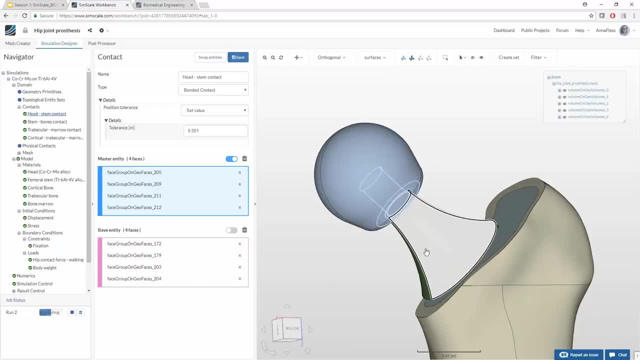 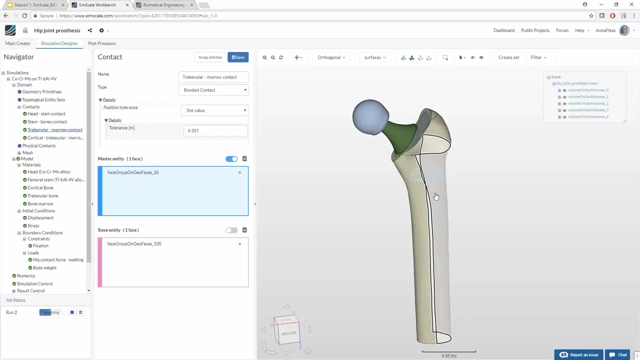 attached to the slave faces of this stem and it's the same throughout the whole, the whole implant. we can see the contacts that have been created. so this is between the trabecular and the marrow, and then this is the cortical, and the trabecular and the marrow are connected. 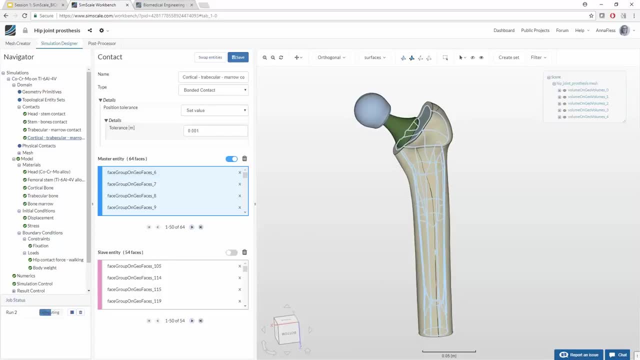 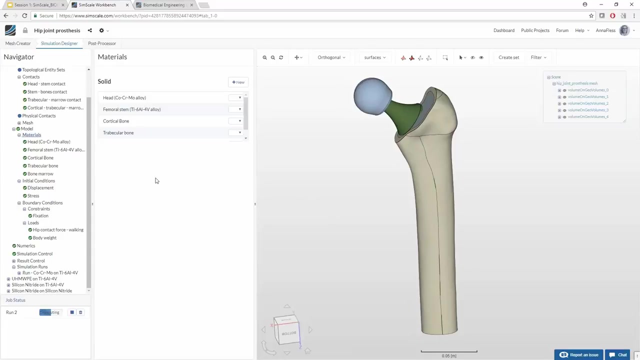 here. ok, so the next, the next step when we go down the tree, is materials, and in this case we're using metal materials. so the, the head and the fem and the stem of the implant are going to be metal alloys, and so the main, the main things that need to. 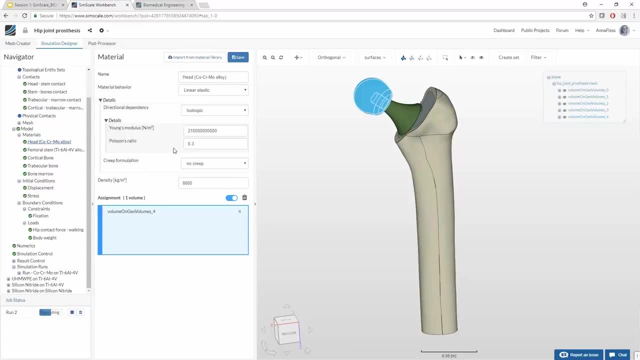 be. The main information that needs to be given in this case is the Young's modulus, which is again the stiffness of the material, the Poisson's ratio and the density of the material. That's all that needs to be provided for the model to be working correctly. 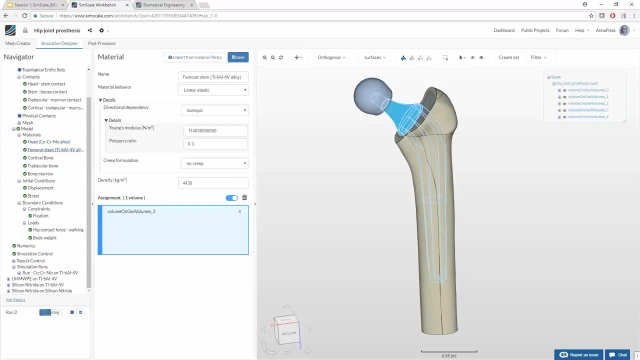 Again, we have to do these. each volume has a different material, so we have to set up each volume separately with the provided material. Once that's done, the next step is we can skip these initial conditions. We don't need them in this case. 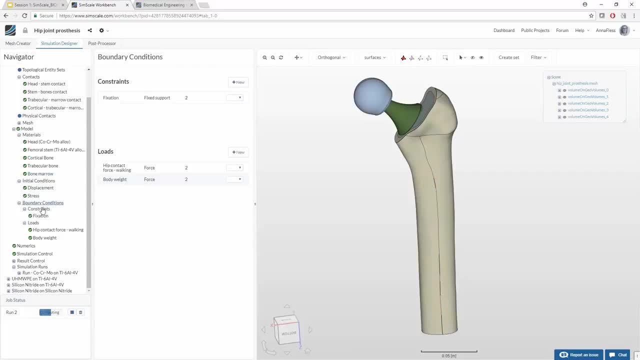 We just can go directly to the boundary conditions. The first boundary condition, as we discussed, is we have to fix this in place. If you look at the bone right now it's kind of just floating. It needs to be fixed at some point. 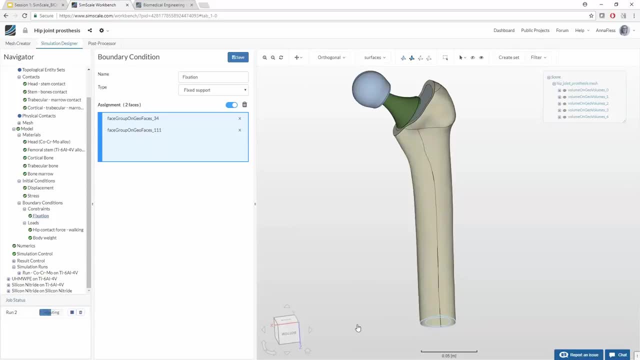 Since we're applying the load at the head, we're going to fix it far away so it doesn't skew the stresses per se, and so we'll fix it down here at the bottom. These two faces will be completely fixed, and so there the elements and nodes there. 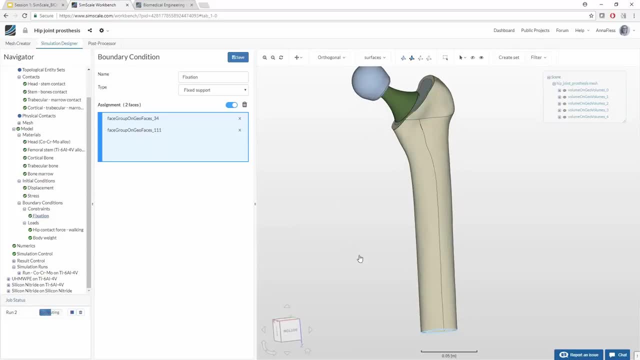 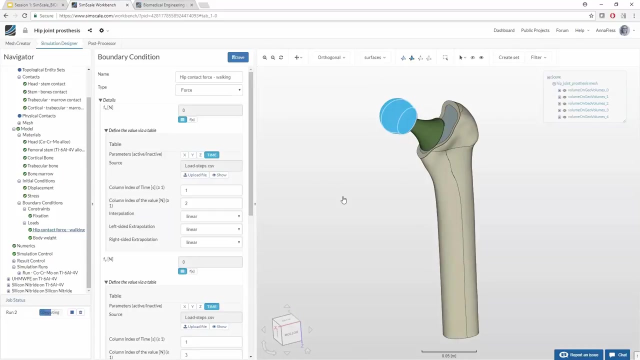 are not allowed to move at all. Now, if we go to the loads, Okay, You can remember that we were applying a walking load, so imagining how the forces are transferred to the hip when a person is walking- and you know, this will vary- 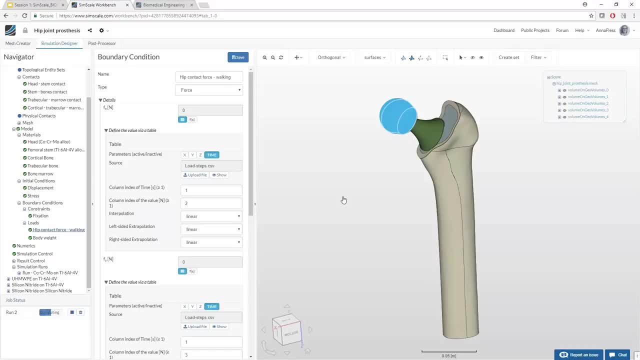 When your foot hits the ground. this is when you're going to experience the largest load in the hip, versus when your foot is in the air. The way this is applied is: I showed you a graph of the variable load, and we can apply this as a table, which is what we've done here. 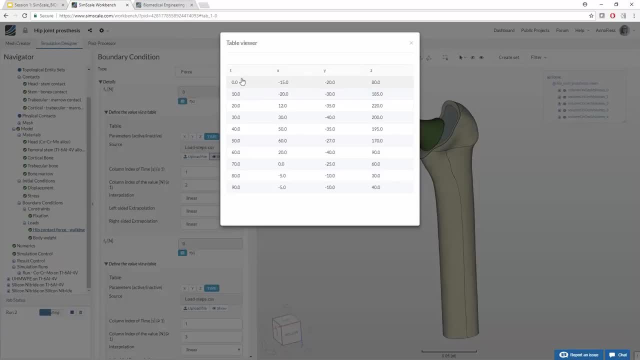 You can actually see we have time, and this is not really time in this case, it's more just different steps. for example, Then we have the load in the X direction, Y direction and Z direction. That's how the variable load is set up. 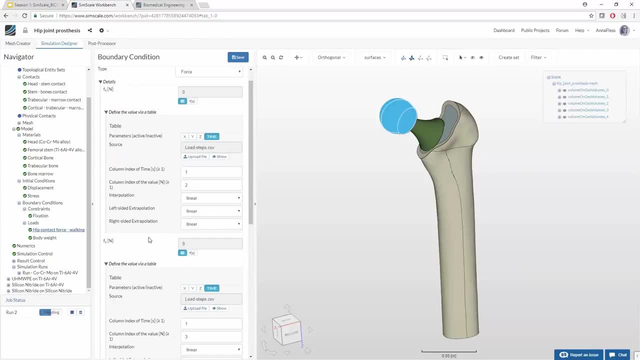 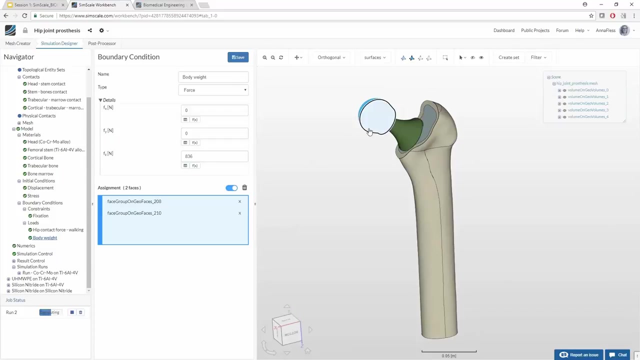 This again will all be explained in very good detail in the homework that I will send you after the session. Then the second load is the body weight load. This is applied in the downward direction. This is just 836 newtons, so about the average weight of a person. 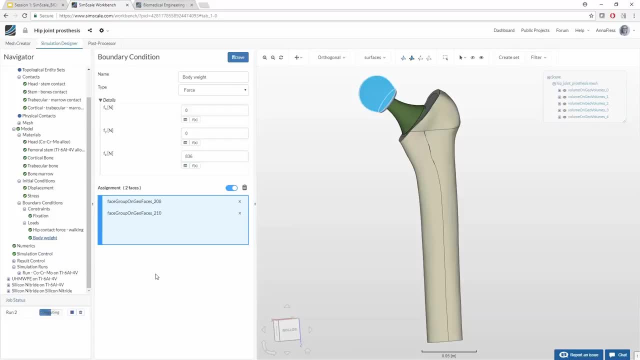 That's the main setup. The final couple steps involve Setting up the simulation, control, number of computing cores and the run time. This example that I'm showing you right now takes about 100 minutes to run, since we want to see how the forces vary on the hip over time or over the time steps that are provided. 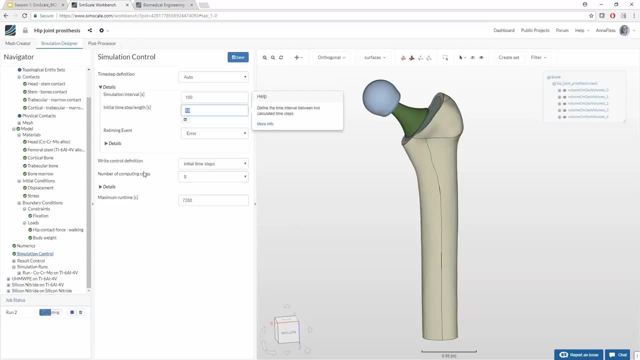 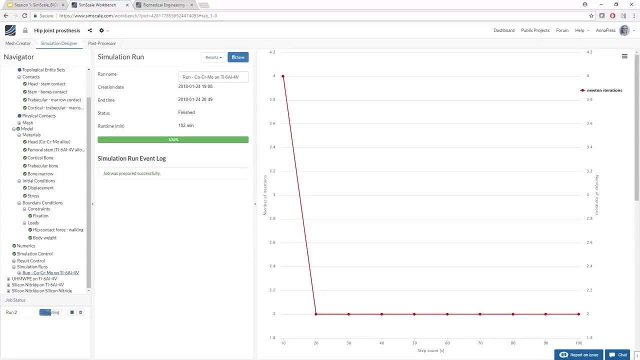 We give an interval of 100, and so every 10 is we'll have 10 steps shown in the final results, And then the last thing to do is run the simulation which you can see I've already done and again, it took about 100 minutes to run. 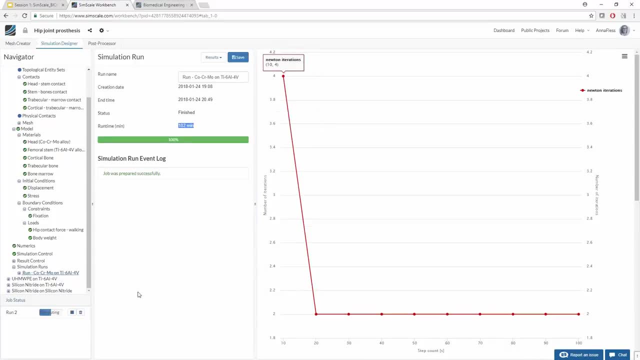 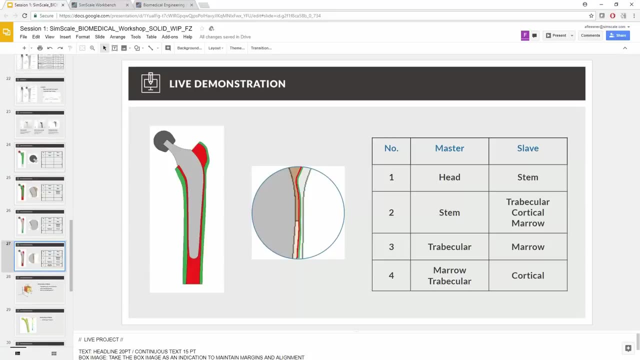 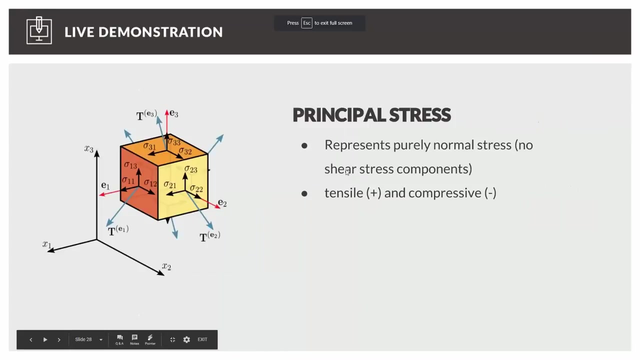 And so that's the main overview in the SimScale workbench of how this works. so I'm going to go back to my presentation and we'll discuss a few things before we look at the results. So before we look at the results, I want to talk about principal stress, and this is 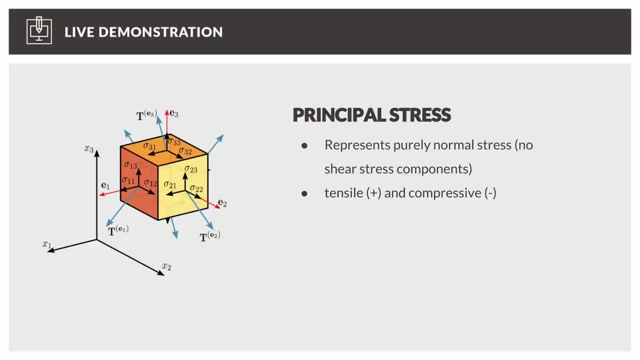 3D, principal stress. So if you see right now we have on this cube, you can see we have nine directions here. And why we're using principal stress is because it shows only the normal stress. There are no shear components. It makes it really easy for us to see where the tensile part of the stress is and the 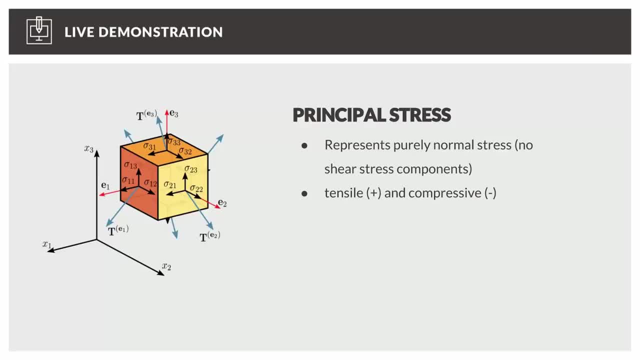 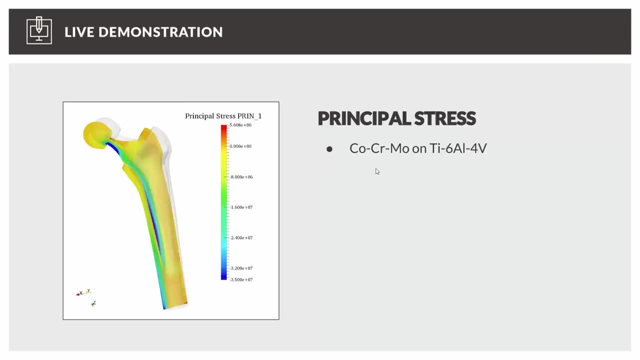 compressive part of the stress is which is what we're most interested in, And so let's first look at these and I can kind of give a description of what's going on. And what we can see in this result is you can see here. let me get the pointer again. 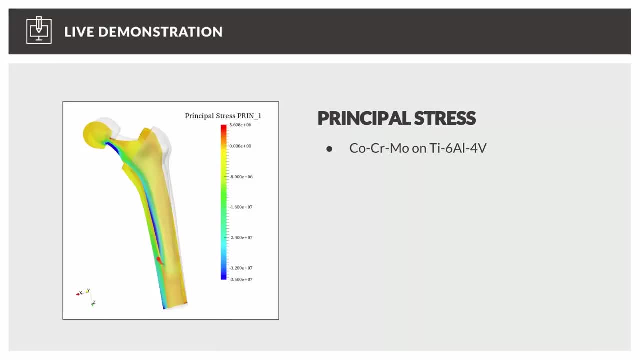 We have the hip implant here and the bone here, And so these are your tensile stresses. The positive is tensile, The negative are the compressive stresses. And remember, on a normal bone we would expect so a bone, a hip, without an implant, we would. 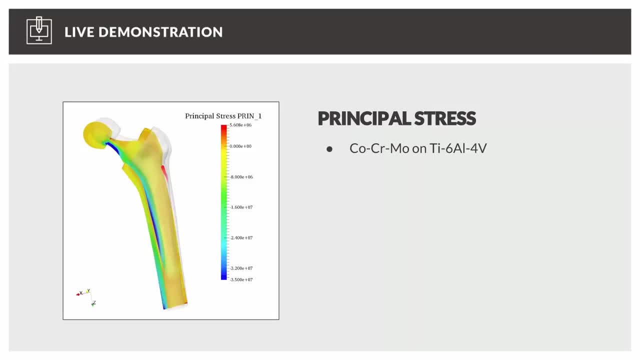 expect to have compressive stress on this side, tensile on this side, and what we see is happening with this implant is that actually a lot of the force and the compressive stress is going into the implant and not the bone. So you can look up here and see that actually the principal stress is very close to zero. 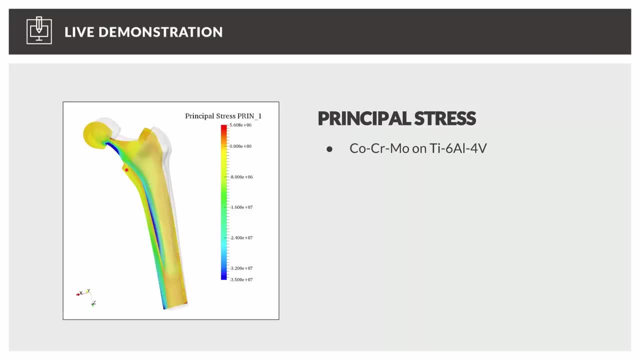 And so there's actually very little load on this part of the bone, And so this was where we'll see the stress shielding is in this region, because this titanium stem is stiff- It's stiffer than the bone And it's actually, you can see, a lot of the force is actually being transmitted directly. 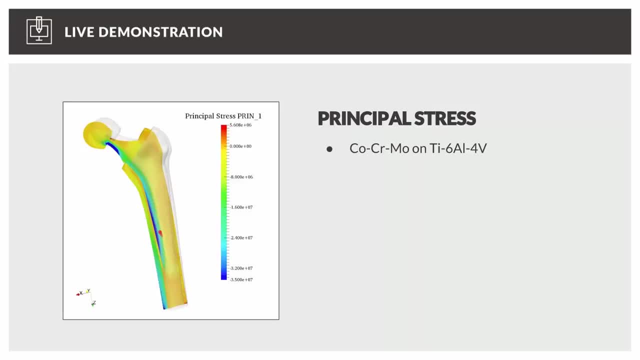 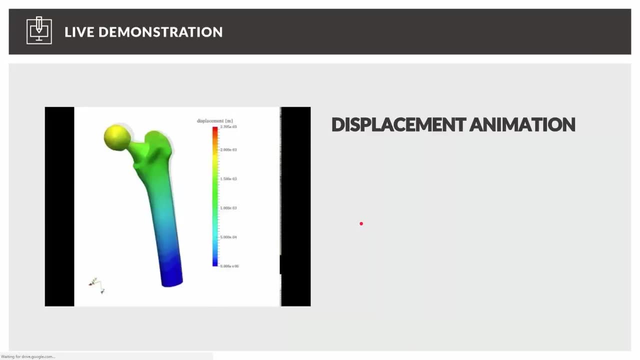 from the head into the stem, And so this will lead to bone loss likely in this region. And the second thing I have is a displacement video. So again we can see over the 10 time steps how the hip is moving under its load. 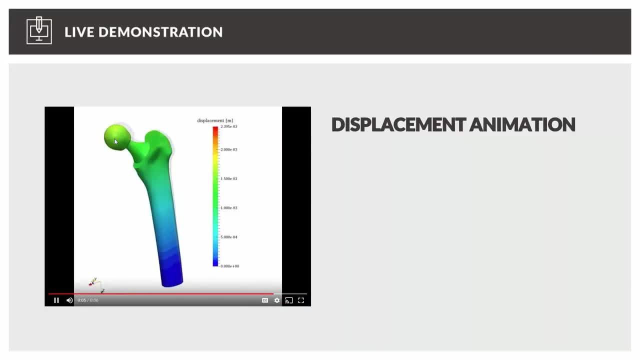 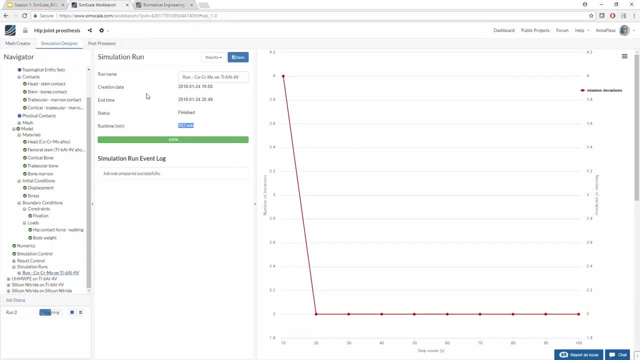 In the middle, when it's the highest displacement. this is when the foot would be hitting the ground when you're walking. Okay, so now we've seen those, Let's have a quick look at how to set that up in the SimScale post-processor. 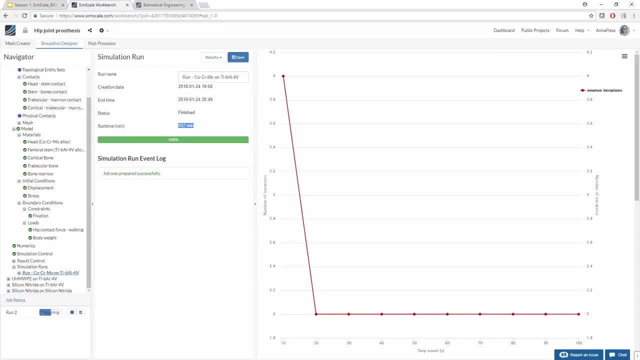 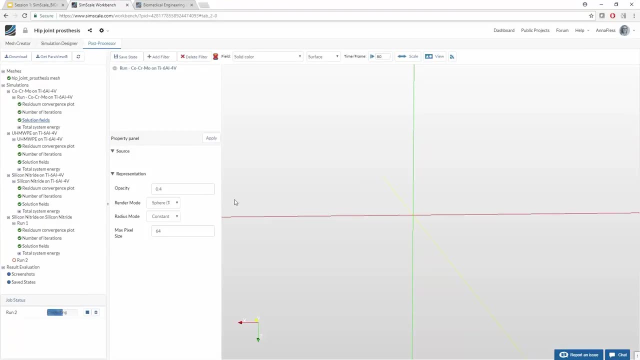 So now I can see that the simulation run has finished. So the last step that I need to take is I need to go to the post-processor, And So in the SimScale post-processor you can basically see the same results that I just 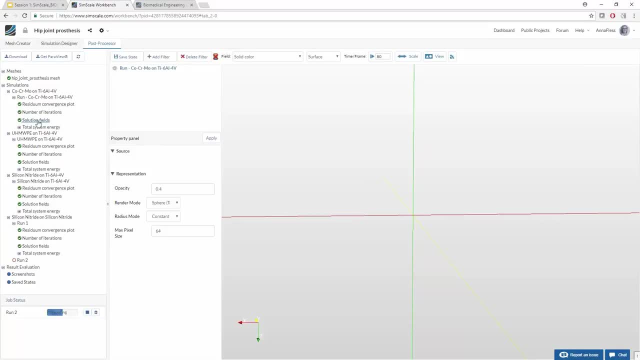 showed you And let me show you how to do that. So I'm going to first click on Let's reset this. I need to click on solution fields. This will take maybe a minute or less than that to load, And once it loads I can see the hip in the viewer. 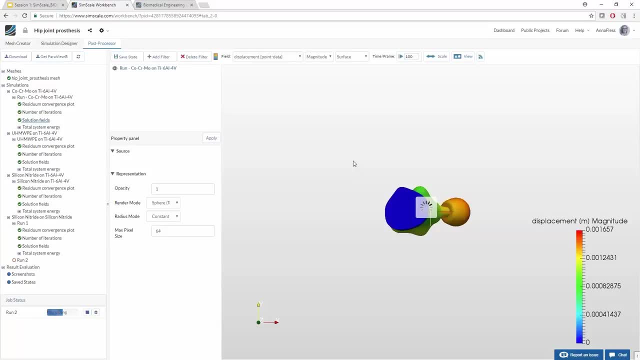 Okay, so let me turn it, And the first thing that I can show you is how to visualize the deformation of the hip. And so, to do this, we can add a filter. It's called the warp by vector filter. Okay, Okay. 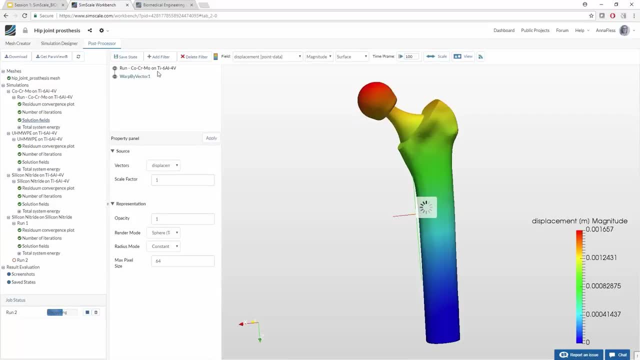 Okay, And now the first thing I need to do is set this to a solid color, With some opacity, so I can see through it. And so this gray, opaque bone will be the, the original location of the bone. And now, if I click on, 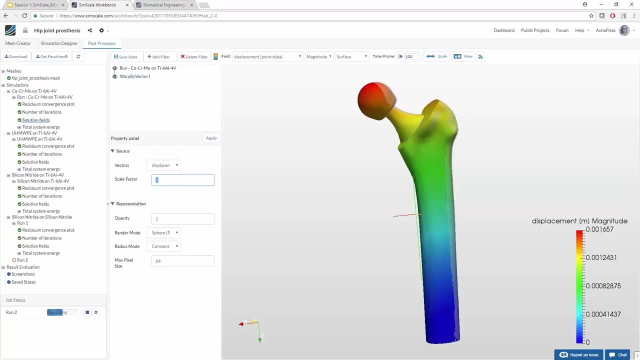 Warp by Vector. I can introduce a scale factor. So now you can see that there's. the displacement is small, which is what we expect. We don't expect to see. you don't expect your hip to displace a lot when you're walking. 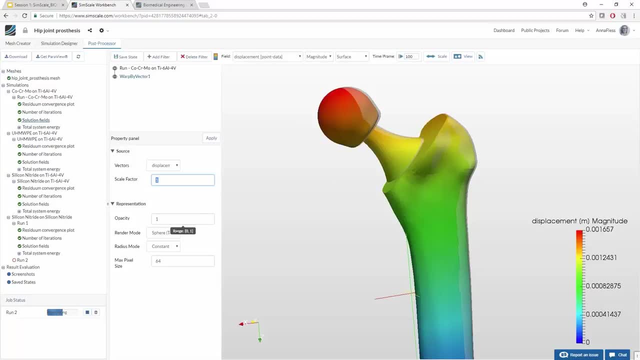 You don't feel any sort of displacement at all. But just to see what it looks like, we can scale it so we can get a bigger view of what the displacement looks like. Okay, So if I zoom out, So now we can see this gray is the original bone. 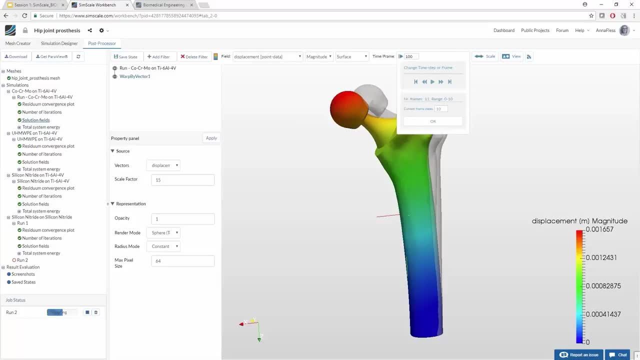 And this is the final position, And I can play this like a video. So if I click play, It sometimes takes a second to load here, But it will start at the zero position And then it will go through the deformation as the person walks. 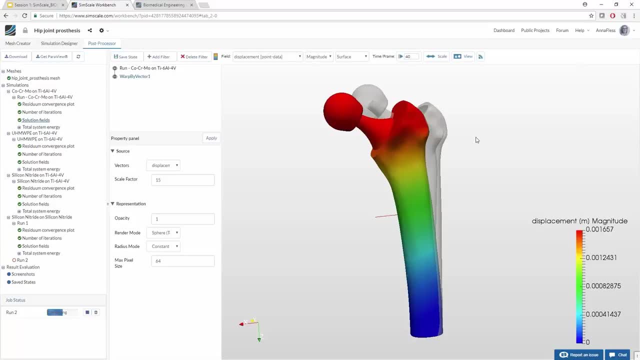 So what it would look like. You can see. the deformation will, the displacement will increase And then it will decrease, And this is how it would be as you were taking a step. Okay, So that's a whole cycle. It goes through, basically, a hundred ten steps, basically. 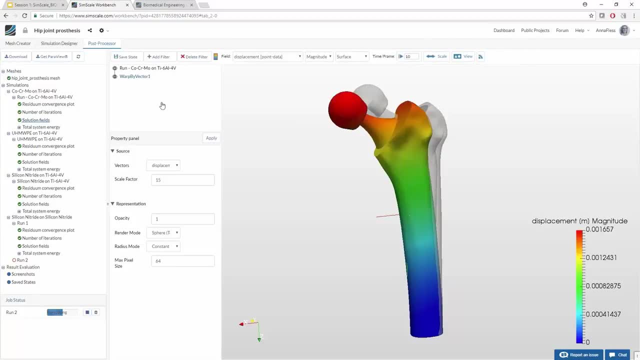 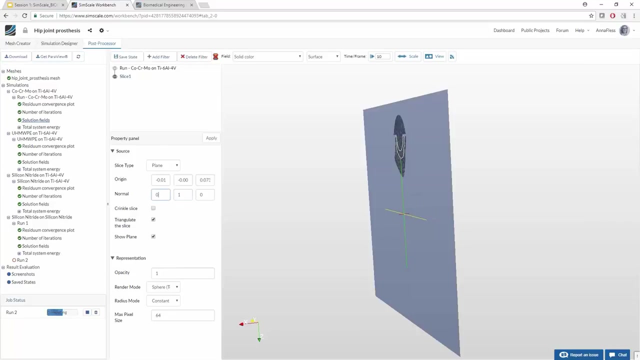 So let me stop that, And I can get rid of this warp by vector filter, by clicking delete filter, And so now we can look at Something else, which is the principal stresses. So let me add a slice And I need to change the direction, so it's in the Y plane. 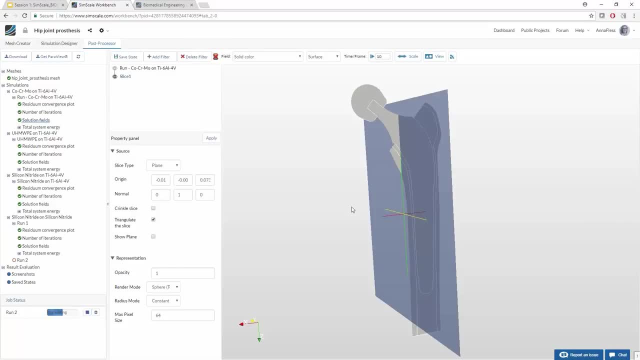 And this is going to give me a cross sectional view of the bone, So in this case I can see the implant As well as the bone in the marrow around it. And so let me change this slice To principal stress, And we're going to use principal stress one. 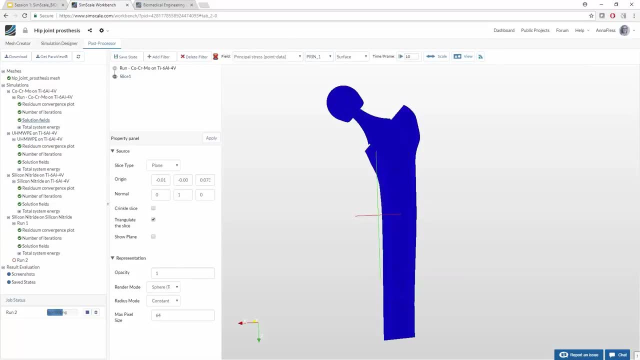 And so this is the maximum normal stress And this is the main component. So these will give me the largest stress, And now I need to set my scale as well. I can auto arrange it, But it's actually. I have some values that will give us a better. 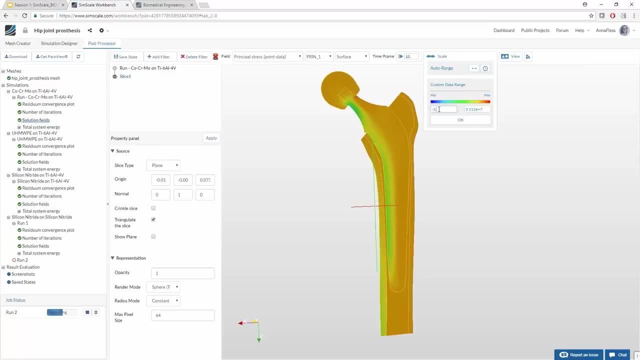 Visualization. So if I put in those values, Okay, So, Okay, Okay, And now We can see. Let me get out the ruler here as well, So you can see the values that are being shown. But again, it's the same. 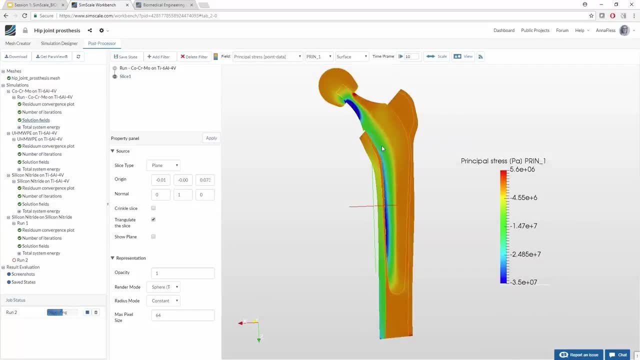 Concept. here You can see that a lot of the compression Is actually going into the implant And not the bone. So up here especially, You can see the very little compression, almost zero, and all of this compression, compressive forces, going into the, into the bone. so again, this is where we're going to see. 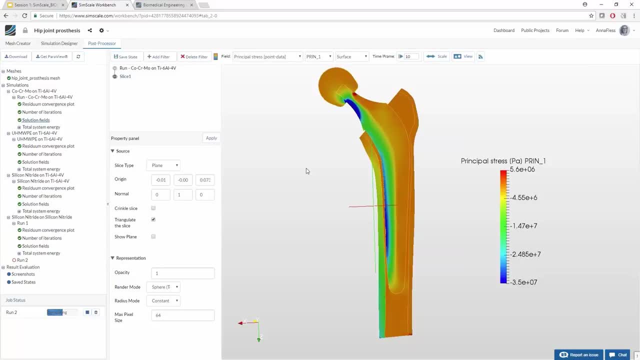 the, the stress shielding, happening and basically what will happen is, if there's enough bone loss, this implant will have to be removed with surgery and then they'll have to do some sort of bone reconstruction before a new implant can be put in. so this is- uh, this is something obviously that biomedical. 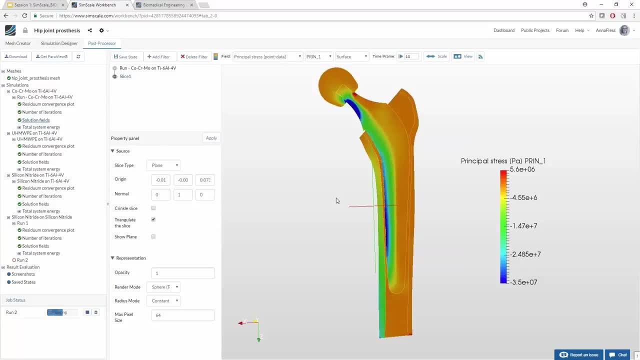 engineers really are working on, because that's very painful for the patient to have to get a hip removed and or a hip implant removed and again replaced, and if this happens every five to ten years, then it's a really a bad cycle. so what biomedical engineers are doing is they're thinking, maybe, about using 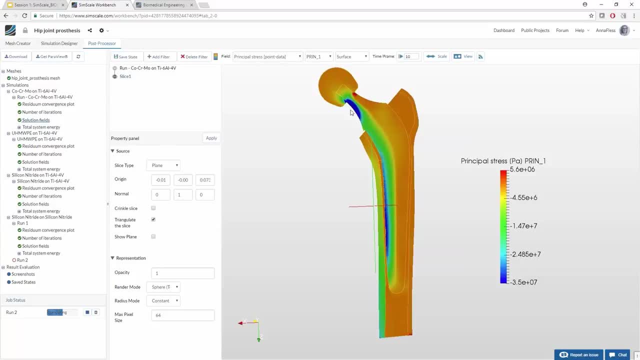 different materials. so again I said: you know this is, this is metal, this is titanium, aluminum alloys. it's very stiff. so maybe if, if we use the softer material, that might be better and allow for more of the force to be put into this bone. and so there's. 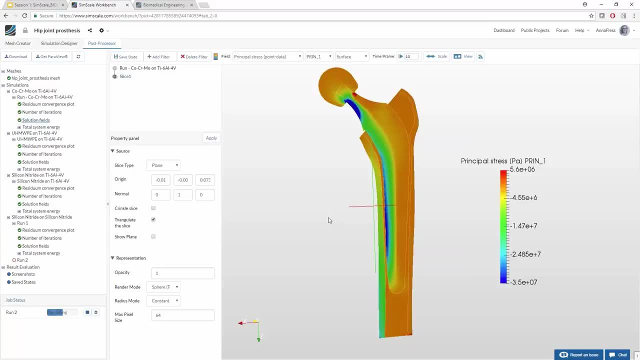 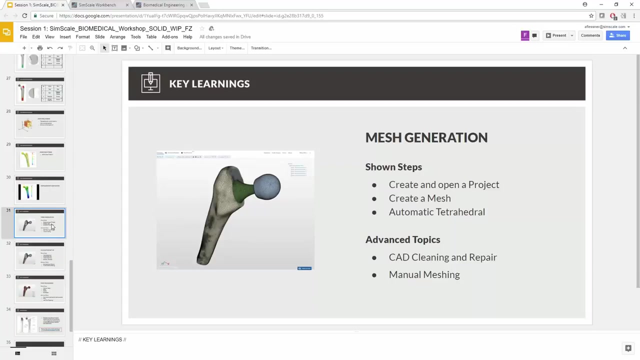 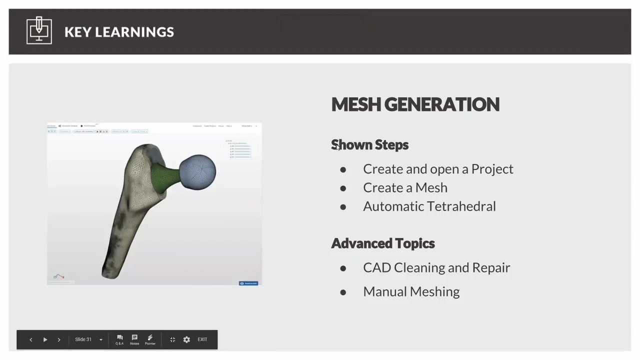 a lot of things that biomedical engineers are doing to research into how they can make this is better for patients. and so that leads me into the final slides of today's session, and that's just to go over what we've learned, the key learnings in this session. so of the demonstration, so the first thing we went, 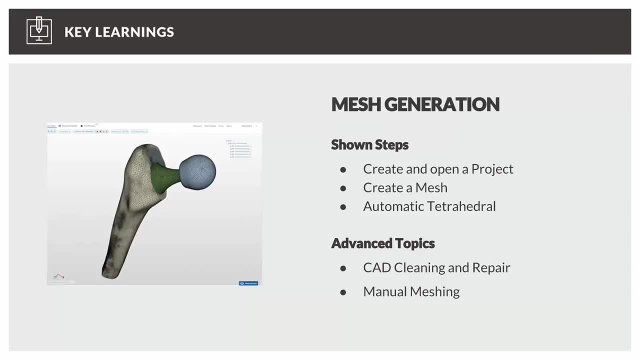 through is how to create a mesh. so it's basically, you're taking the, the CAD model that was uploaded, and breaking it down into smaller tetrahedrons, and this allows us to solve for the stresses and strains on the hip. the next is the simulation setup. so we created contacts, we assigned materials. 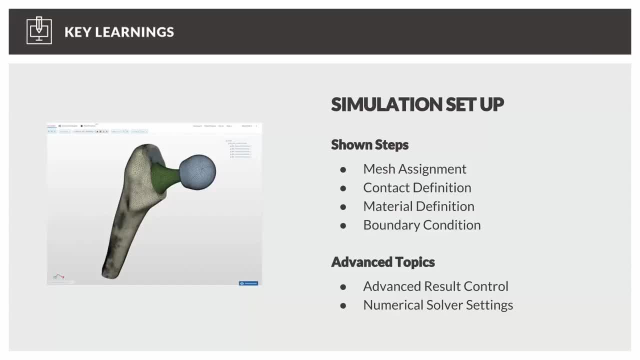 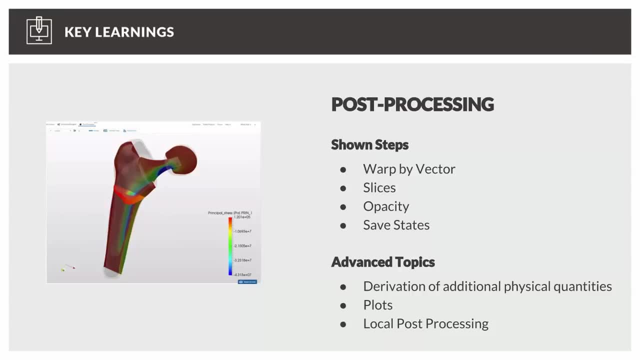 to their respective volumes and then set up the boundary conditions. and then we went through and did the post-processing. so we looked at warp by vector so we can see how the hip is deforming. we looked at a slice so we can look at how the principal stresses are acting on the, the bone in the implant. 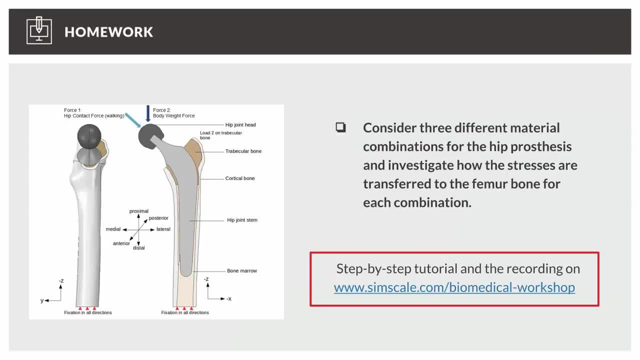 things like that, and that leads to the final slide of this session, which is your homework, and so, like I said, biomedical engineers are constantly maybe looking at new materials or designs for a hip such as this that will work better and create less bone loss for the patient, and so 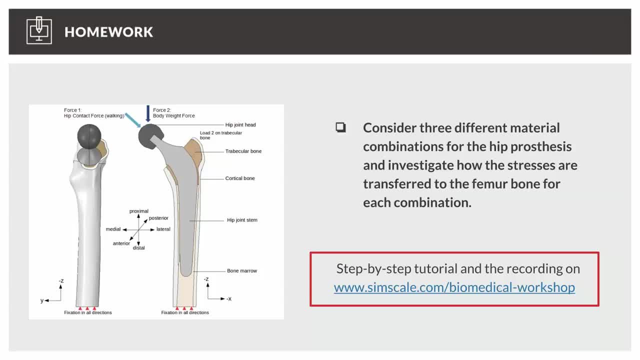 what you're going to do is you're going to consider three different material combinations for the hip prosthesis. you're going to look at this first combination that I just showed you, that's a metal head with a metal stem and, as we, as we saw here, this is a very stiff implant. the second combination that 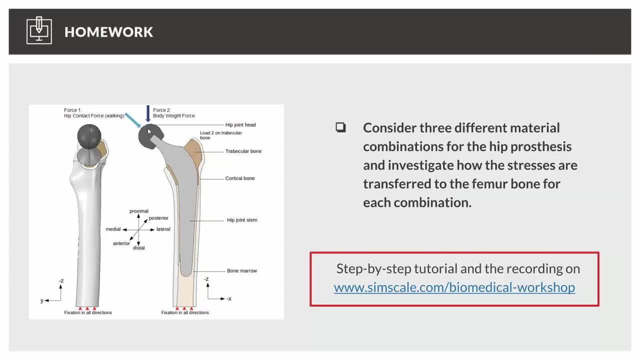 you're going to look at is a plastic- high, high weight plastic head with a metal stem, and so this, this head, will be less stiff, since it's a plastic, and sorry about that. and the third combination that you're going to look at is a ceramic still, or ceramic head and stem, and so this is less stiff than 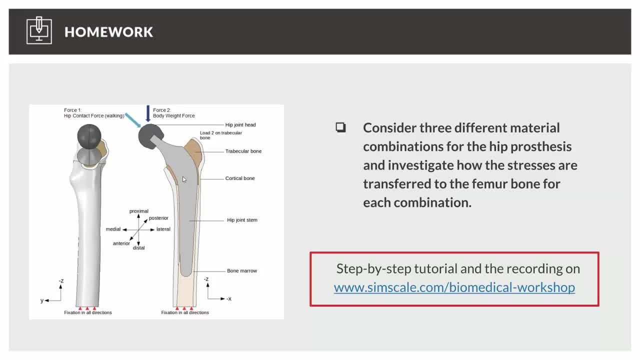 metal, so maybe you'll see a difference in the load that is going into the, the implant, compared to the bone. so this is what you're going to investigate. the step-by-step tutorial and the recording can be found on the biomedical workshop page. i will send you an email that has this, the recording of this session, as 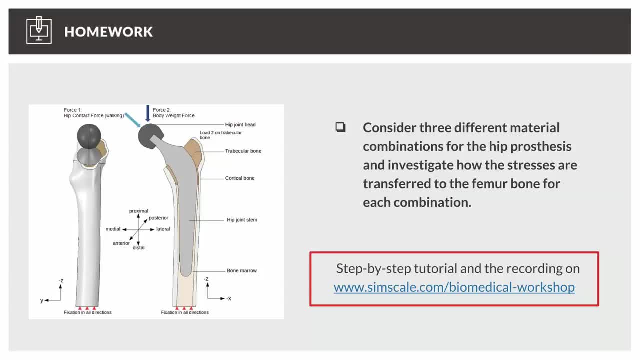 well as a link to the homework in it, and so you can do this over the next week and you can ask any questions that you might have while you're doing the homework in the forum. we have staff that are very active there that will help you, and so I hope you you learn a lot along the way while you're doing. 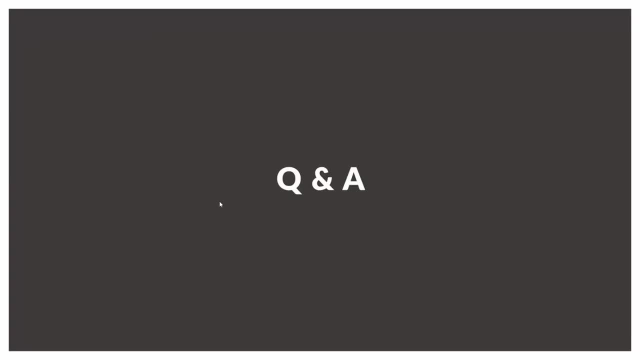 this. so that kind of wraps up everything I want to close. it looks like there are some questions from users, so let's go through those briefly. um, let's see. so Antonio asks: can you briefly explain the process with repairing geometry for meshing? how difficult is it to repair? so, Antonio, this will depend on your model generally. 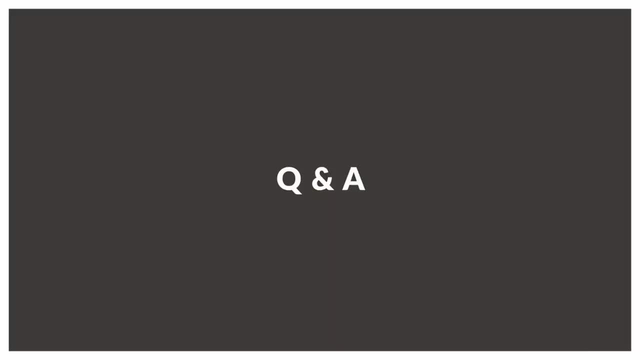 you want to. so, for example, if we have, you know, in this case you could see the surfaces were all very cleaned and the contact was good between each volume. so you don't want to have basically separations between faces, you don't want to have small. so, for example, for another- you know- finite element case, maybe you have like. 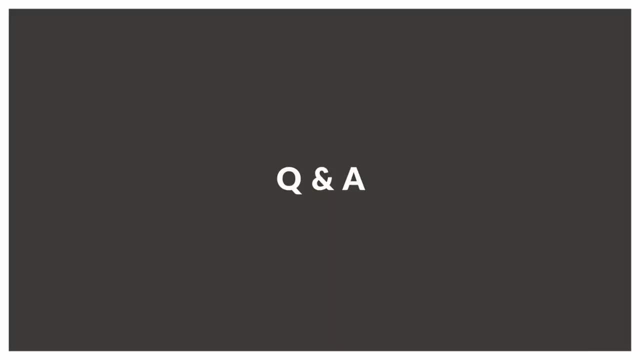 an aircraft or something that has very small bolts on it, or like a bridge, if it has these very small bolts and if, if, if these don't really affect how your simulation is running or where you're going to look at the stresses, then you should remove them from the model and just put a simple, you know, flat face, or 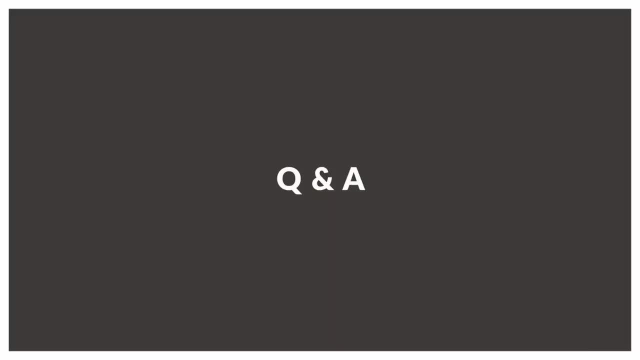 fill, fill. take out the bolts and fill, fill in where the holes would be. so it makes it easier. basically, the measure will have issues if you have very small faces or geometry problems like that. another question is: what are you using to reprofile the human bone? so I think 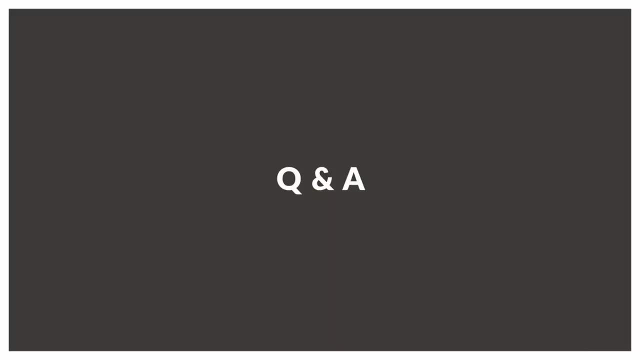 this bone was actually taken from grab cad, so I'm not a hundred percent sure how it was created, if it was scanned, so that's that's kind of a question I was going to ask for to see. cannot answer for you on that, sorry about that. are there any other questions? 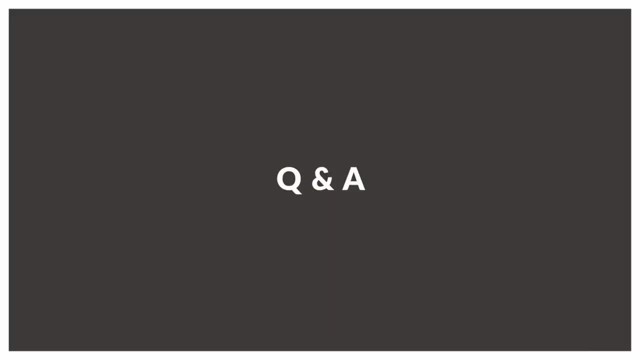 okay, it looks like there's some more. so fjords asks: is it necessary to include marrow into the model? the contribution of marrow to the mechanical strength of the bone is small and removing it would allow the model to solve faster. I think you might be right here. I don't know how much faster it would solve, but this is. 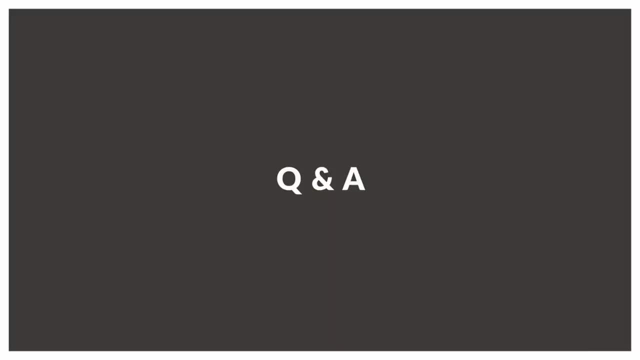 kind of the finesse of doing FEA. you have to decide which- and this is kind of you know- differing opinions. it depends, you can test, you know both ways and see if your results are the same, and then you, then you know that maybe you don't. 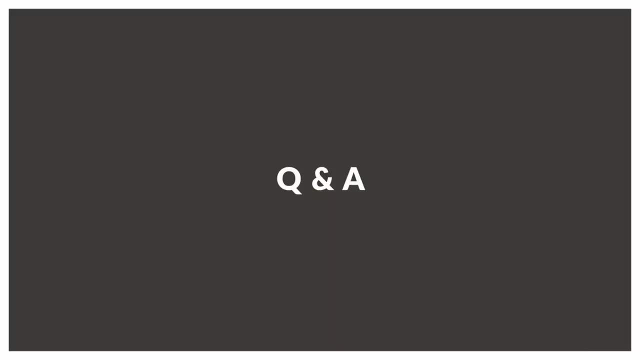 need to model the marrow. so you- yeah, I mean this is something that maybe you could explore while you're doing the, the homework- if you take out the marrow and notice that that the results are different. but I mean another thing is you have to remember the, the. 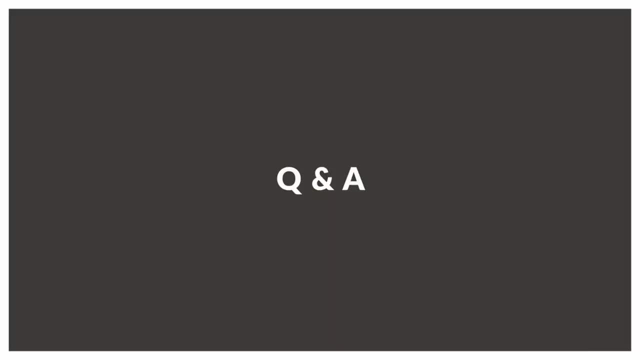 stem needs to be in contact as well. so there, yeah, there, there are definitely different ways to to model every case and you can kind of compare how the results are and what actually needs to be modeled, what's important in the model and what is not so important. 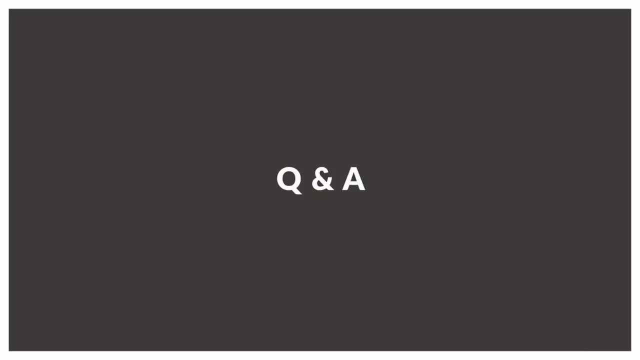 to each of these different types of models. you know you do the DE کو and just start to see it's. that is, they can interact and using reasoning, and so your models train you to see the different types of models and then test them. so, at the same time, I think, if you're the project manager and you know, 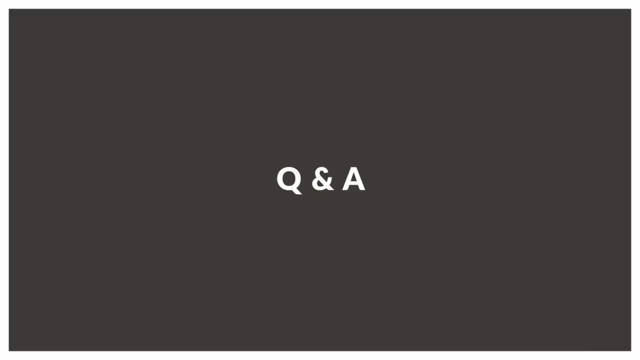 I'm And who's going to be doing all this and want, if we have a our natural environment when they do this process it's. it's not going to be only on me, but you're going to find instructions on how to do that in the SimScale viewer. 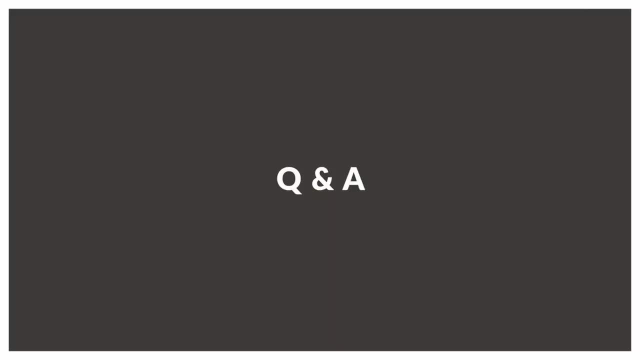 Basically we can use a transform filter so we can put all three different designs in one window and we can compare the results. So you'll do that during the homework. Okay, Carlos asks regarding processing or computation capabilities available with SimScale. 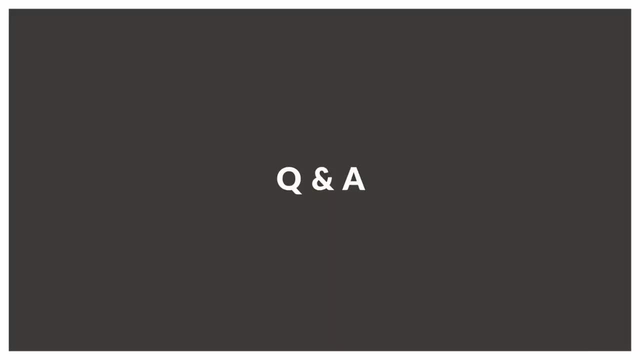 you used eight processors. Could more be selected to finish sooner? This is also kind of a complex question that you would have to do some testing, because what you have to remember, Carlos, is that you know, say, instead of using eight processors. 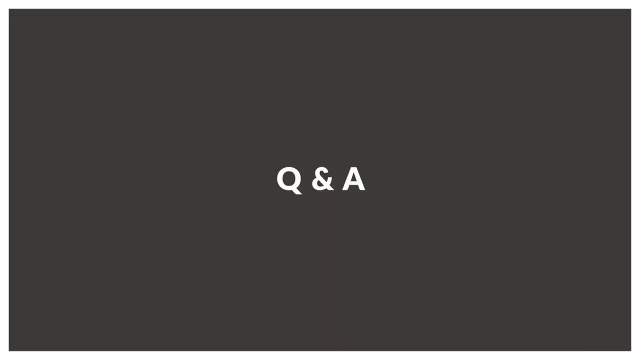 we use 32 processors, And so what you're doing is you're using some of those processors to compute everything in parallel, And so it depends on, first of all, your solver. Is the solver set up? Is it set up to be run in parallel? And also for a relatively small problem. if you run a lot of processors in parallel, maybe it won't finish faster because those processors need to communicate the information to each other, which also takes time. So you need to scale the number of cores that you're using based on the size of your mesh. 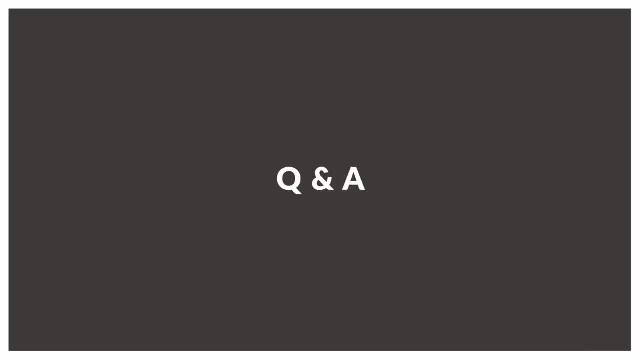 Okay, let's see. And Gustavo asks: where were the material properties of bone marrow obtained? So we obtained all these values from a paper, and that paper is cited in the homework, if you want to have a closer look. Okay, I think that is going to wrap everything up. 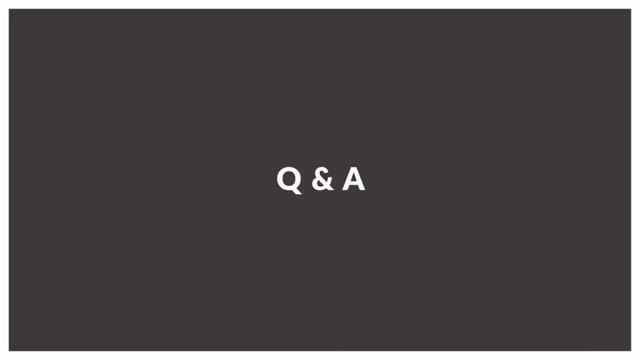 I don't see any more questions. So I thank you guys for your time today and I hope you enjoyed the session, And I will send an email out tomorrow with the homework and the recording so you can have a look and get started on that. 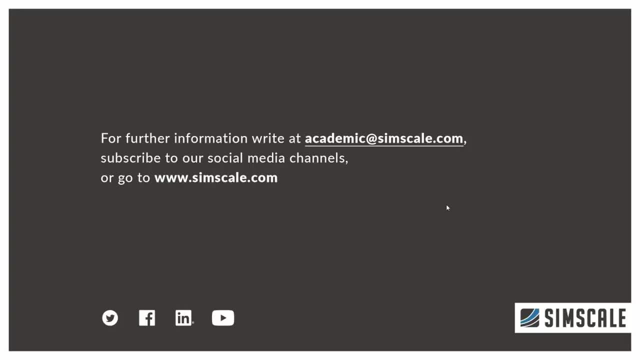 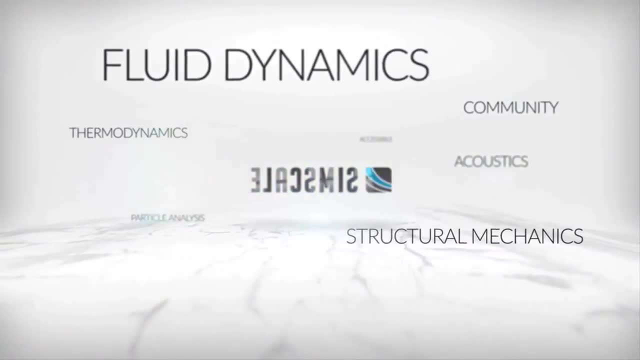 So have a good night and I will talk to you later. Thank you.